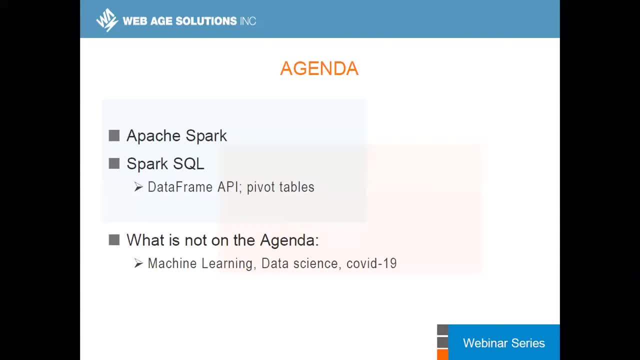 So we feel that there is a big demand from business community, from business analysts, from people who are data practitioners, who would like to use something fast, intuitive, resembles SQL And which would enable you to process data on a large scale. So today's presentation will be recorded and it will be published later on. So, if you 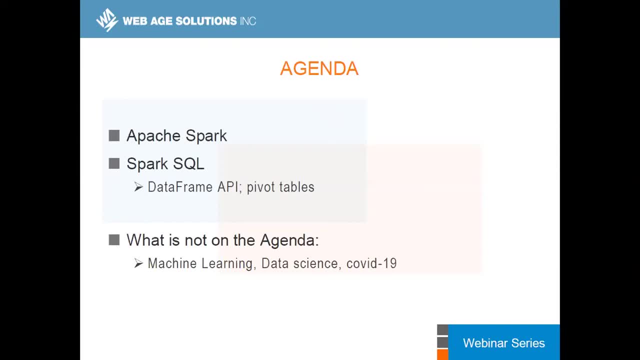 would like to download it. you can do it later. So it looks like we've got quorum, So So, So, So, So, So This presentation is targeting the not kind of programmers, Even though you, you can have a programming background, you can. you can be a data engineer, you can be a software engineer. But I guess the primary focus is on how to make Spark, or more specifically, Python on Spark, to work for you as kind of a. 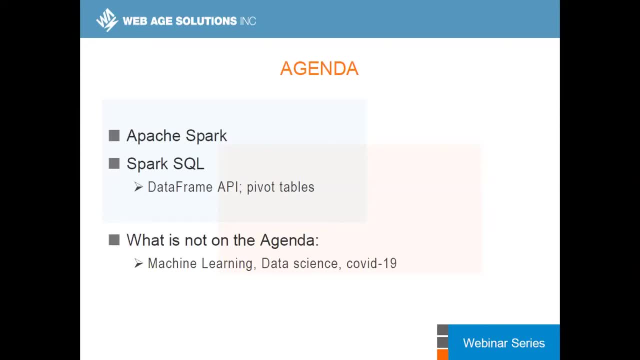 Python on Spark to work for you as a kind of a sql like interface, and that will what would be the uh- the main, i guess uh- topic. there will be some discussions around some other points and it looks like what's happening what we see in the field is that people um, um, exploring and going into the area of processing big data on a cluster. 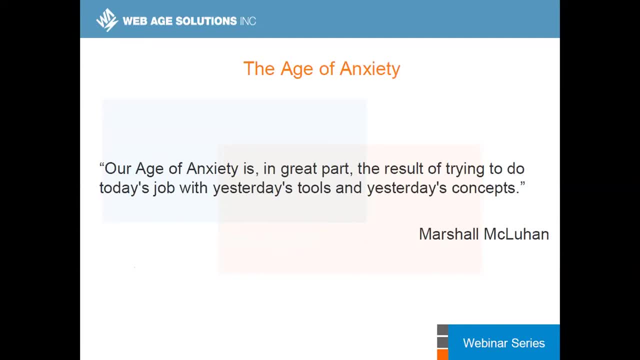 of machines using a variety of systems, like hadoop gives you apache, hive or empower uh similar systems that you can find, but at the same time, um uh, you can uh just observe that more and more people are using spark. uh, it plays very nicely, it's just, it's very nicely integrated into the. 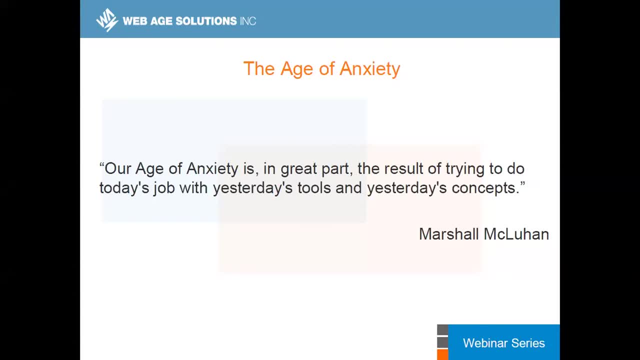 hadoop product ecosystem. uh, it works against hdfs, it works against other types of storage, um, so, if you have any questions as we go, uh, we are not able. uh, you, i want to be able to enable your, um, your voice questions. but if you would like to put your question, 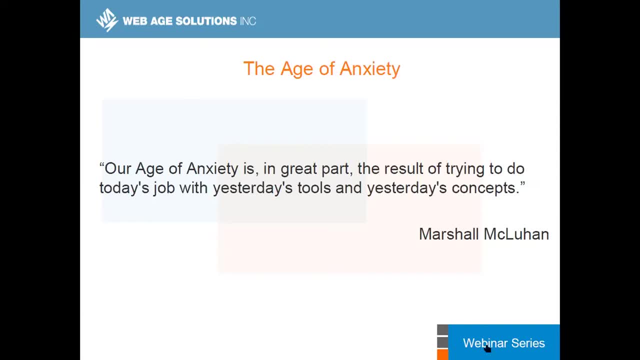 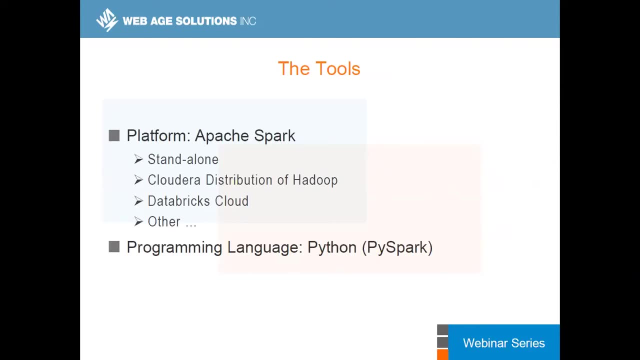 in the chat window, feel free. so uh the tools, uh, the toolbox. um includes uh, papa spark and python. so those are the two things that you need to be familiar with in order to take advantage of um, of that sql like capability that is available um to you, um on this platform, apache spark. 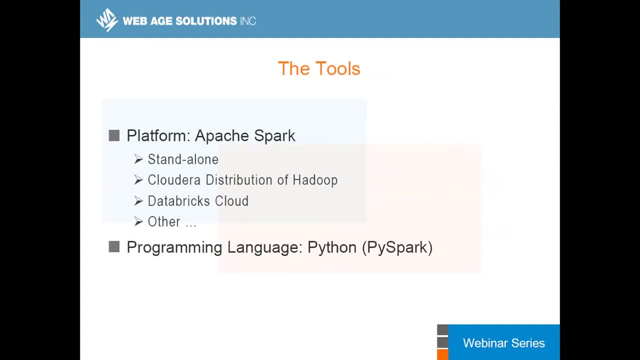 is an open source project, as you can judge by the apache in the name, um. you can download standalone spark, but you are better off to use um, um, cloud error distribution of hadoop or cdh, which comes with all the hadoop products, the main products used on hadoop, including spark. unfortunately, spark 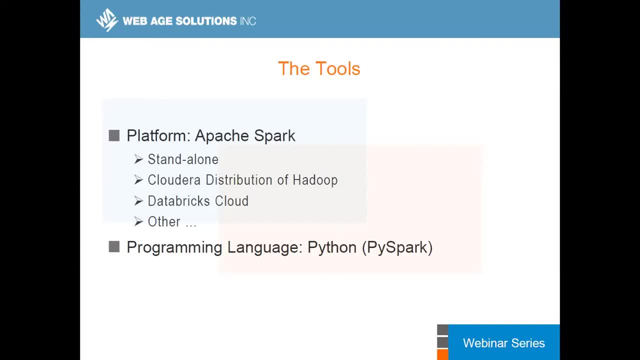 might be a little bit dated- uh, not, maybe the latest 2.4, even version 3 now- but it's very well integrated. it can read the hive meta story and get very nice integration with hdfs. also for experimentation you can use databricks cloud. that is a community edition a little bit scaled down, not enterprise grade. really there are some. 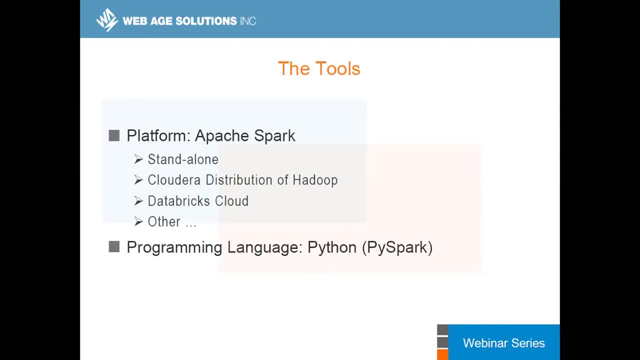 limitations as to the number of cpus, virtual cpus, which will be allocated, an amount of memory, the size of data sets that you can produce uh provide um databricks uh use. by the way, that databricks is the company which was formed by the original developers of spark, so they know. 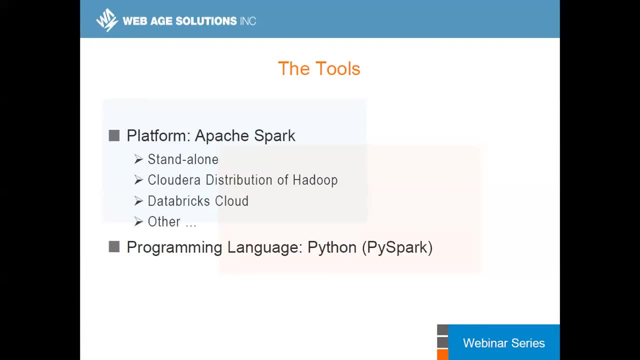 their their material. databricks cloud is based on amazon web services and the focus in today's presentation will be python. even though you can use scala, you can use java. some people even use r, but r is more limited to standalone and databricks cloud. it's not very well integrated with cdh. 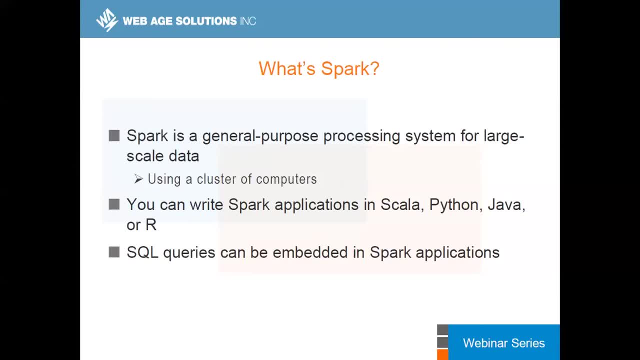 so quickly. uh, what uh is spark? uh, i don't want to preach to the converted. if you know what it is, just bear with me for a couple of slides. so spark allows you to process a massive amount of data which is stored on the cluster of computers. so essentially, uh, it's kind of a hadoop, uh, but but. 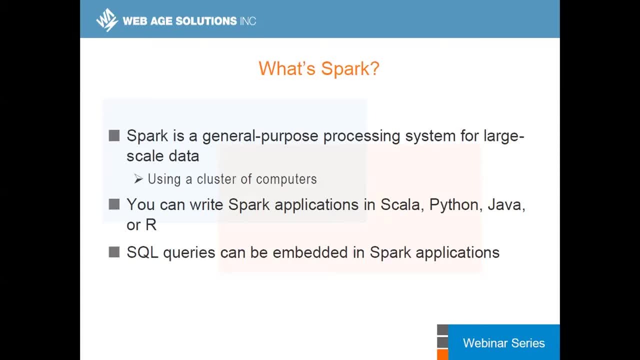 much faster. if you compare uh spark with the map reduce engine, it's several orders of magnitude 2 or 3 um faster. uh, it's just almost near real time um. you can interface with spark as a platform using your expertise in the languages listed here. so the consensus now is to use uh scala for mission critical um applications where you. 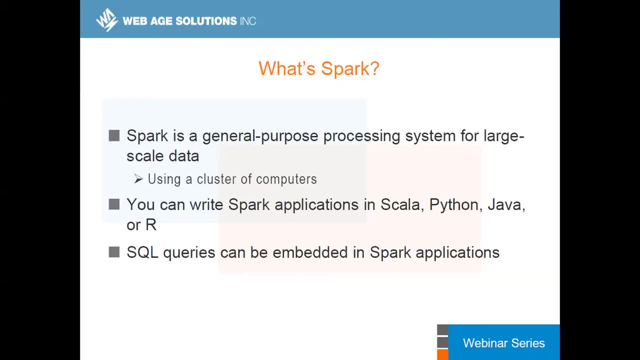 really want to get squeeze every ounce of performance. uh, java, probably just losing to scala in terms of the concise syntax and, um, very compact api. uh for data science, machine learning. even though those are not the topics, we've already published a number of webinars um on this topic: machine learning, data. 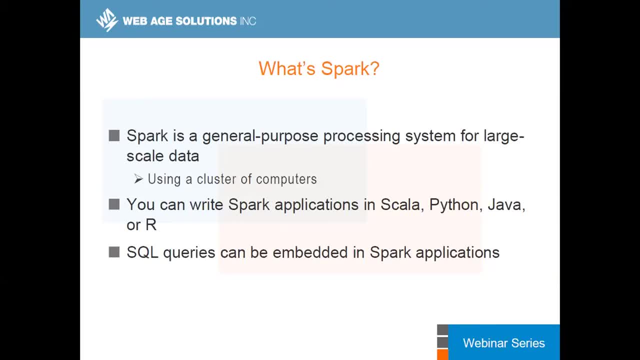 science, state engineering, uh with, uh, using spark. and here we are just looking at again at um, the Spark SQL module which gives you access to SQL like interface to the underlying distributed data. So the main advantage of Spark is that it tries also to lure people from business side of the world of the organizations to use SQL queries. 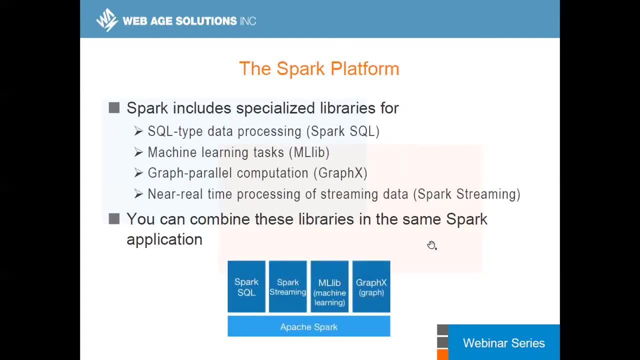 which can be embedded. So Spark platform. it's versatile, quite rich in terms of functionality You can have. you can find libraries for solving your machine learning tasks, processing graphs and near real-time processing using Spark streaming. but the focus of this presentation is Spark SQL. What's 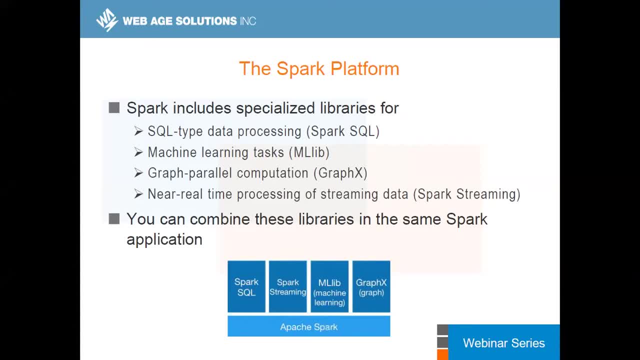 interesting about the platform is that all those modules- they are integrated across the Apache Spark platform, meaning that you can ingest data through the Spark streaming endpoint, which is sort of like socket server. data is streaming in, captured in real time, and then you can apply machine learning algorithms on the fly. 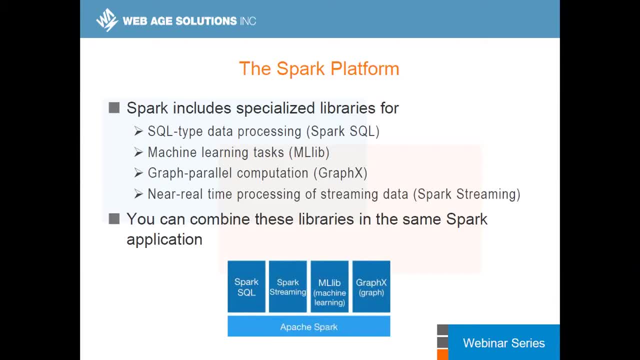 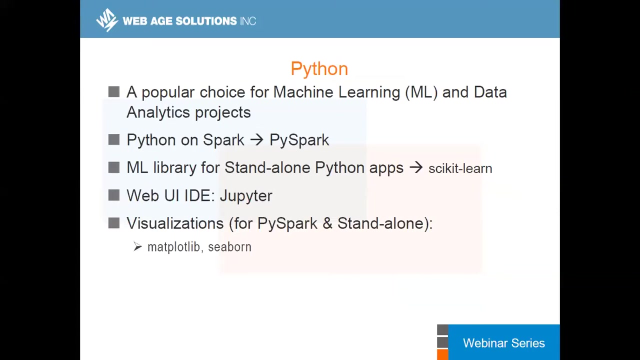 Right. Spark SQL is no different, but you are better off to process data in batch mode, So that you have ingested data, data is sitting on your cluster at rest and you would like to process it to get some insights, So Python. so I mentioned earlier that the tools of what most people have started using 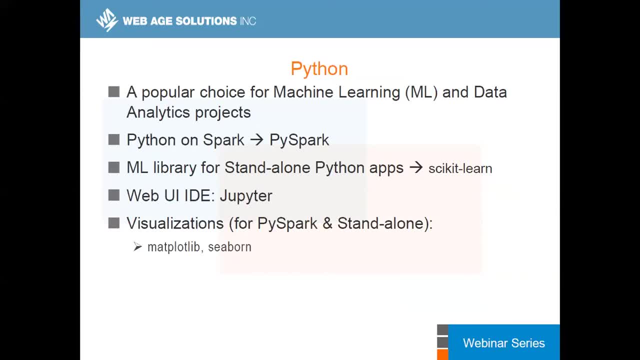 and that's where I guess people are coming together to use Python. Python is a very popular language now. you can find it in various parts of the IT landscape. You can use standalone Python and standalone Python running on your laptops. You can use scikit-learn. 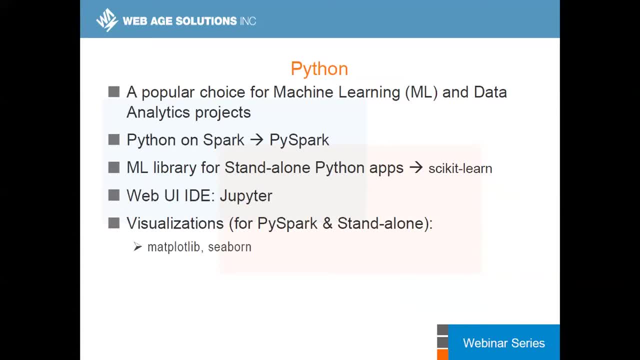 for machine learning. Python on Spark is the regular Python which has been augmented with libraries and interfaces through the Spark platform. It's called PySpark Python on Spark. Python is also nicely integrated with modern integrated development environments, including Jupyter, and it has very nice production-ready visualization supports. such libraries as 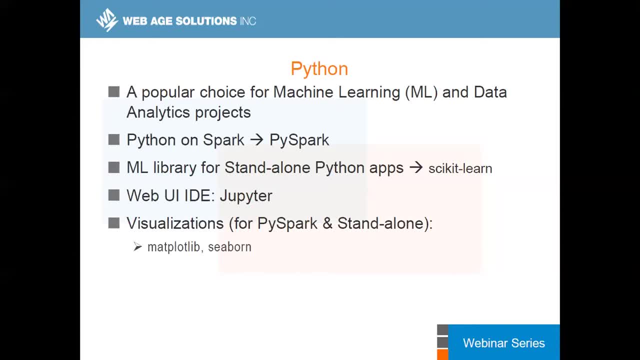 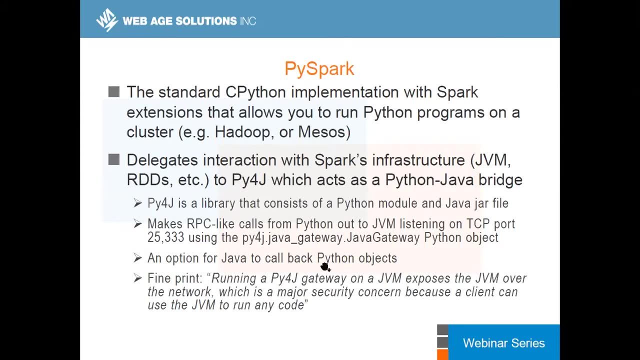 SmartPlotlib and Logic Engine Seaborn, based on Matplotlib, give you very nice and free visualization capability. So PySpark, it's a little bit noisy slide, but it just gives you a little bit of a background so that you understand it's regular Python. 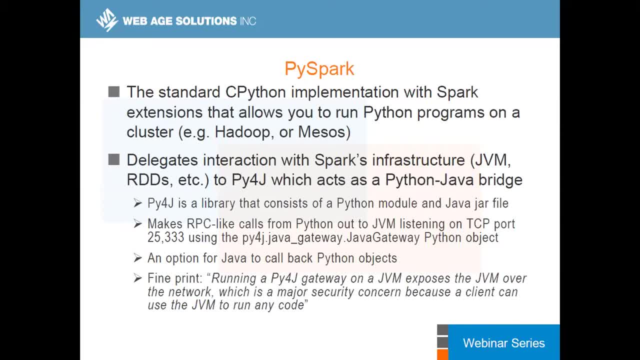 It's has been implemented using CPython implementation And when it runs on the cluster machines, particularly on Hadoop, it uses JVM. So Java virtual machine needs to be present And there is the RPC library which sits between Python and Java. 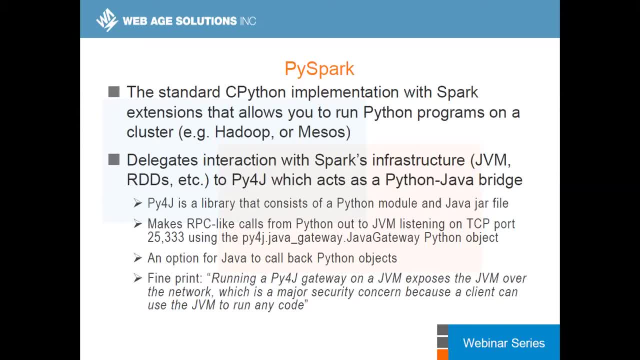 So you might say that it's kind of be very restricting. but in fact Python is pretty much kind of a dispatcher. It just sends the requests to Java and Java actually performs all the heavy lifting And Python just provides wrappers around the objects that are turned through that RPC. 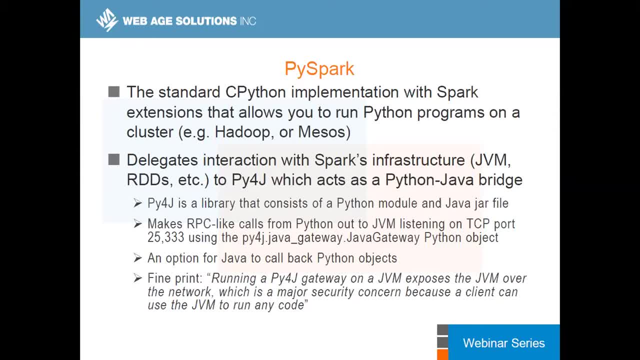 remote procedure: call bridge. Okay, so you are not losing very much, other than the Python itself probably is not as performant as you would expect from other languages like Java, And Scala is definitely a better choice if you really have mission critical applications or applications where every second or minute. 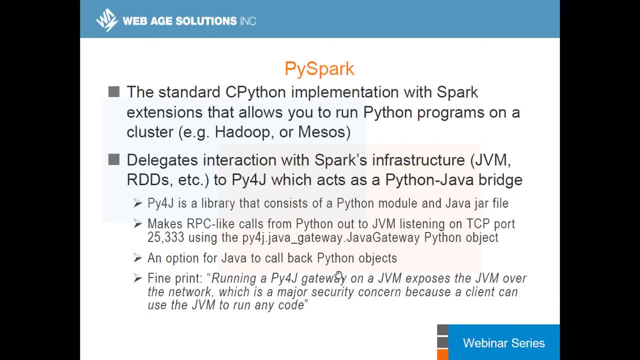 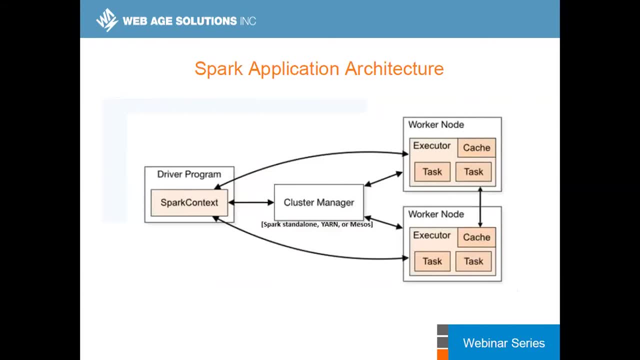 of processing time counts, Python would be a little bit lagging, lagging behind, And probably it would be the last. a couple more slides about the Spark. So is that you understand that things are being processed on Spark in a distributed manner? 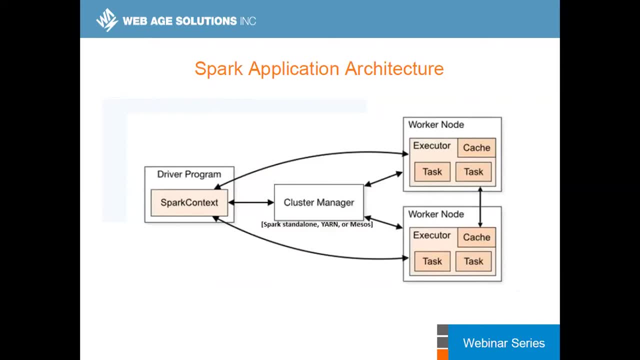 You've got your data sitting on 128 machines and belonging to a particular logical file. It's just been partitioned as if it was file allocation table and you will be able to process the data on all those machines. So there is a this distributed processing model. 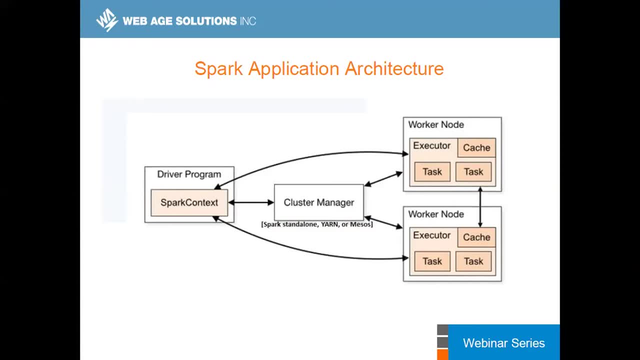 like scheduling of tasks to run on the cluster of machines working on that piece of the data, that split of the data, segment of the data. So there are some concepts that you should be familiar, like the executor and the driver. So driver, essentially it's entry point to a program. 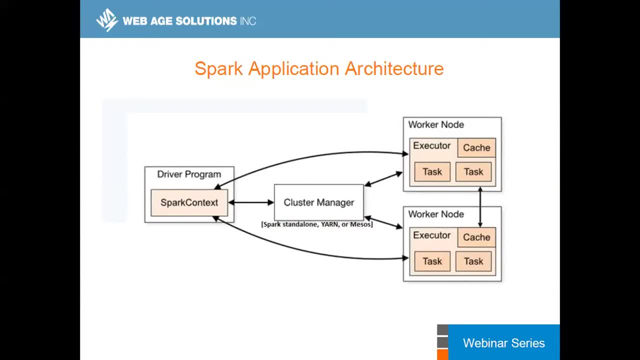 It's public static void main. if you're familiar with Java or Scala, It's the main entry point and you create Spark but context, which is an object interfacing you with the rest of the system, And then you will be going through the cluster manager. 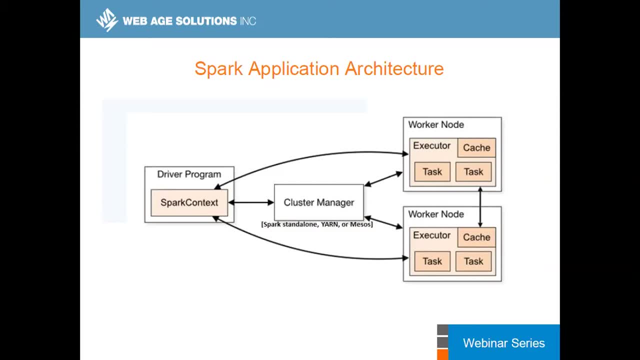 of sorts, be it Spark, standalone YARN, which is Hadoop or Mesos, And the executor is a JVM plus Python runtime which works together in that RPC bridge. Spark tries to solve all the tasks in memory without really discussing executor problems. 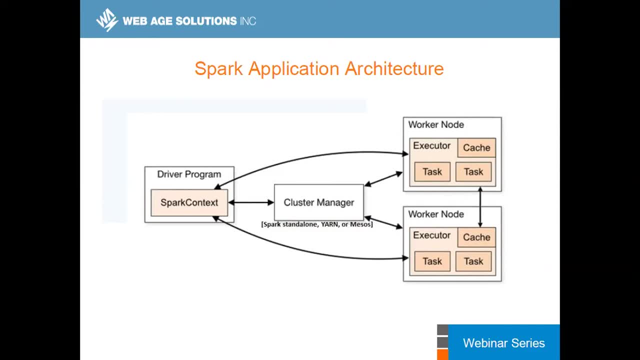 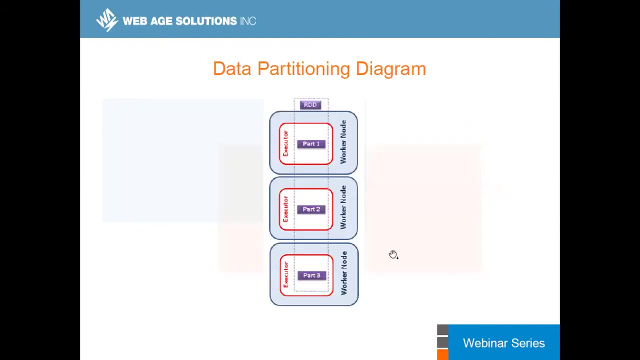 It tries to use as much as possible aggressively using caches. So those tasks can be anything. It can be a specific task for selecting data or filtering. It can be map reduce as well. So if you say you've got three parts of your data sets, 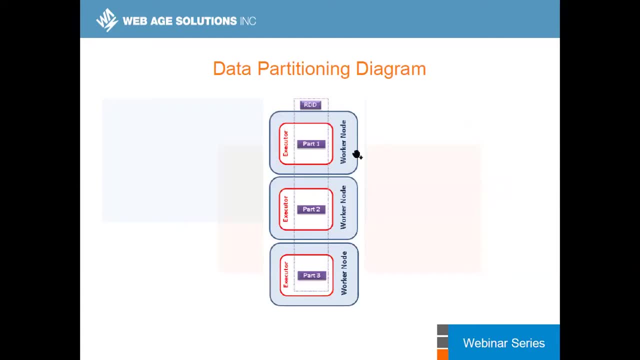 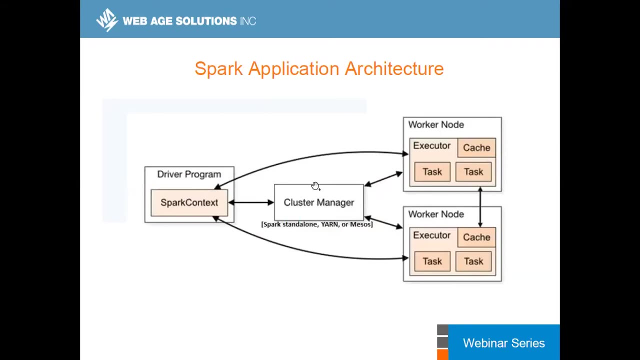 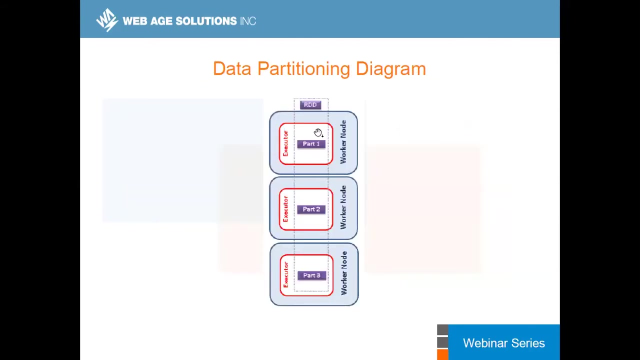 sitting on three machines, So there'll be three executed processes allocated by the cluster manager, and the driver program will actually be driving through the application manager to make sure that every block of your data is processed in sequence And the output pretty much you've got. 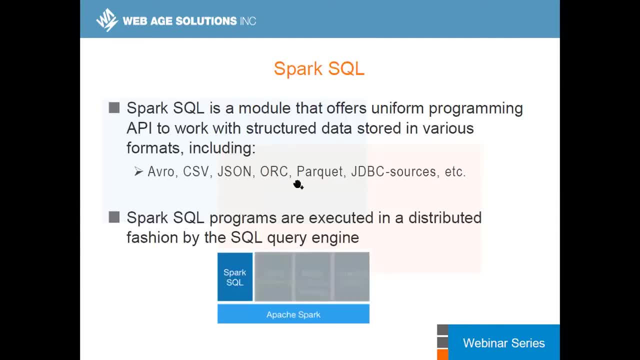 three threads of execution. Okay, so that's pretty much it to set the background. So now we understand that Spark gives you all the mechanics that's necessary. So now, what about the API? In order to take advantage of the SQL, the memory? 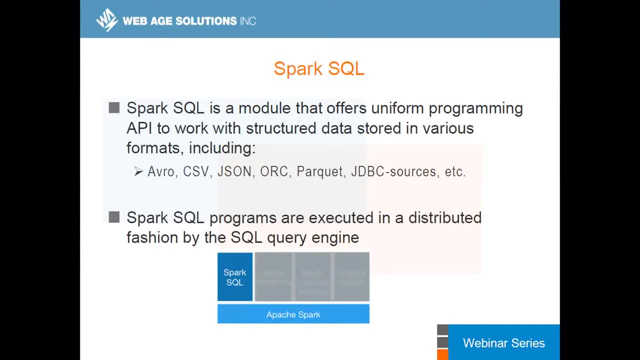 the embedded mode and more. you should use Spark SQL. So everything is already integrated. You don't need to do anything extra other than just initializing the interface to the Spark SQL module. What's interesting is that Spark SQL, even though it sounds a little bit limiting. 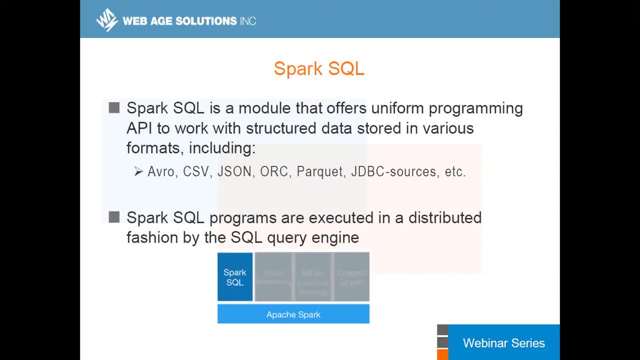 that SQL probably is not enough. So I can get SQL from Oracle DB2 or Postgres database. But the thing is there are many other ways to do this. First processing will be done in distributed manner. Again, thousands of computers. 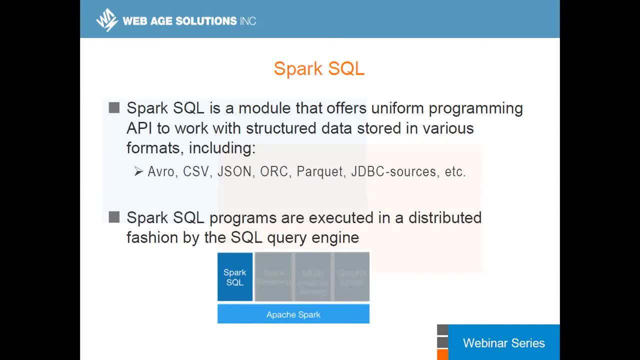 hundreds, tens of computers can be involved, enlisted in processing your task. That's one thing. The other thing is that Spark SQL offers you uniform programming API to work with a variety of data stored in distributed manner, So your data can be in any of those familiar to you standards. 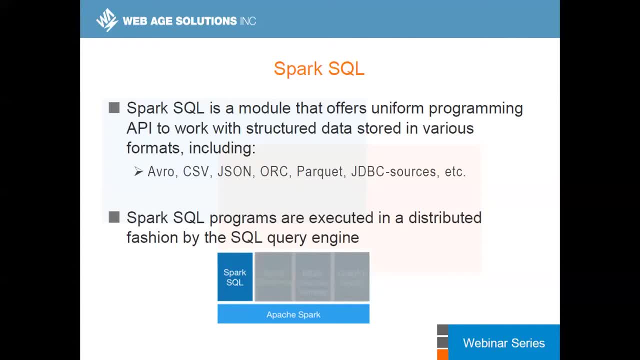 like CSV, It can be in JSON. But in addition to that it also supports Avro, which is very popular on Hadoop. It's kind of a serialization format And columnar stores Parquet and ORC, which are very efficient mechanism for storing data. 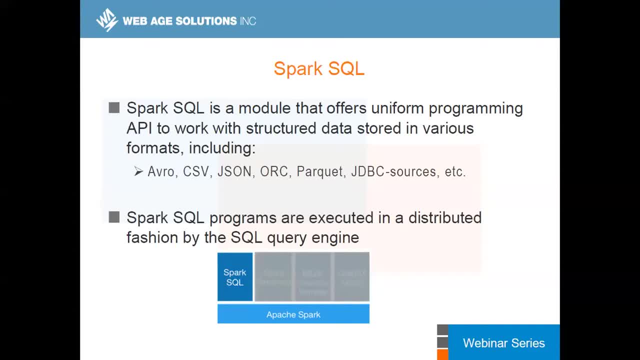 and for data retrieval. You can also connect to available JDBC database, JDBC enabled And there is a JDBC driver which would allow you to pull the data out of a specific database, bring it into Spark, process the data in distributed manner. Probably it'll be a little bit of a overkill. 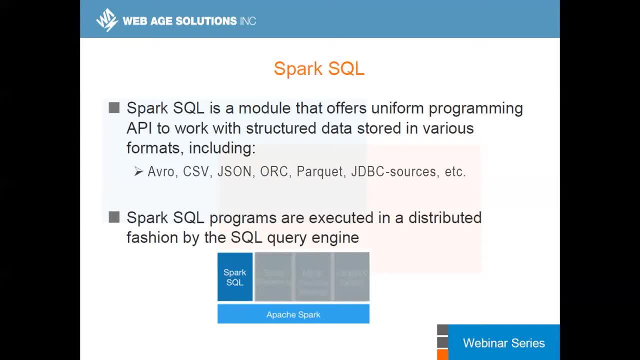 It's not a very popular thing, but still you can quickly prototype certain tasks and probably compare some time. If you run a similar query on the target database and then it downloads the data source, can you pull all the data from a particular database? 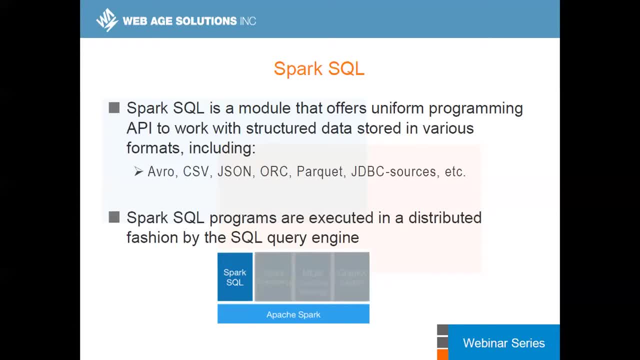 from a particular data and you start processing it using Spark. Of course you don't have the ability to take advantage of indexing, clustered indexes and whatever is available on the database side, But there is no, I guess, limits as to how many machines could be involved. 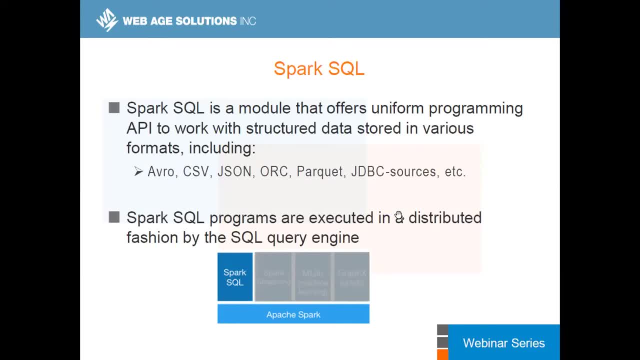 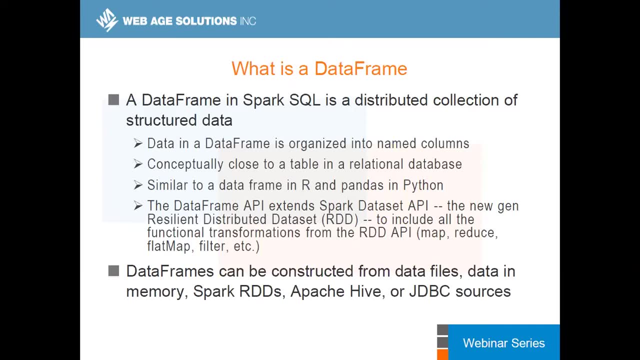 So that's, I guess, the context. That's the big picture where things are. And now let's go right into what Spark SQL is about. Spark SQL is based on the data frame. It's the fundamental storage, in-memory storage construct. 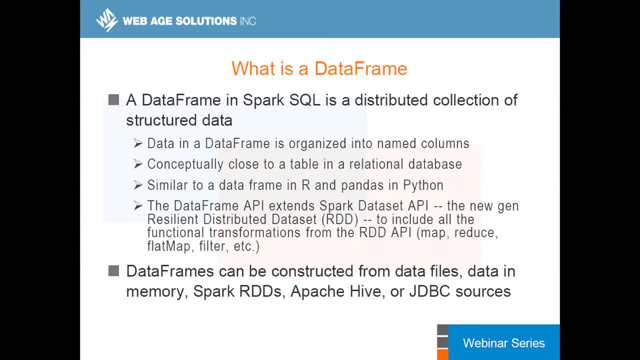 It's an object which allows you to wrap up in a logical way distributed collection of data. Distributed means across cluster of machines and all the coordination of the processing. dealing with failed nodes, restructuring and eventually doing some optimizations to circumvent certain steps is done at this level. 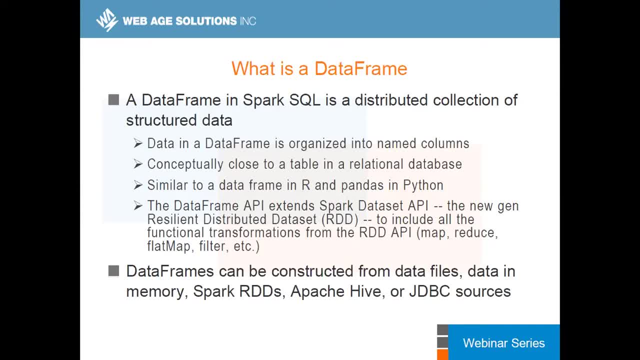 So data frames- if you are familiar with R, that's where I guess they got that name upon this. Essentially, it's very close to a table, the concept of a table in a relational table database, Data frame API. it's just newer, a new generation. 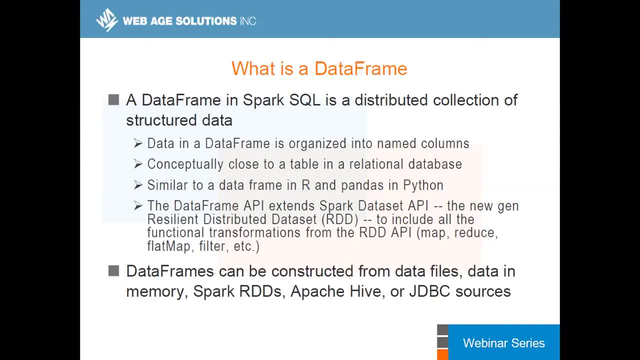 and it's based on the structure or API, which is based on the low-level RDD type of API, So RDD. there were some iterations with RDD getting the data set kind of a facelift, but data set is type-specific. 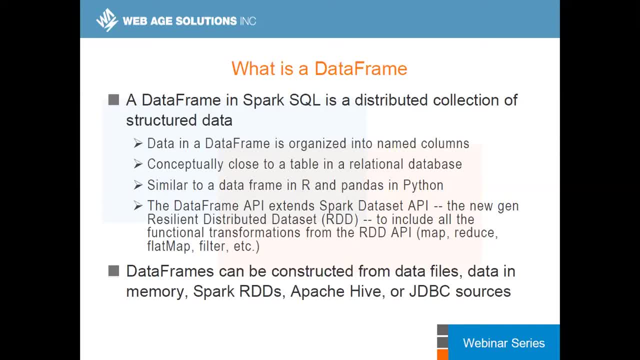 It's a strongly typed system and only Scala and Java can take advantage of it And data frame. essentially, it just creates a uniform structure. It's a very simple structure, a uniform wrapper which would allow Python to tap into that underlying data set API right. 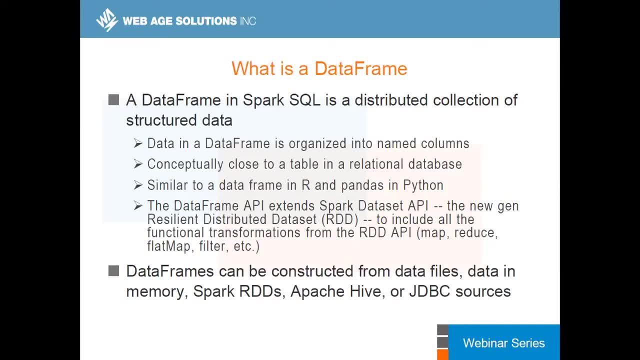 Also, data frame, in addition to exposing SQL-like API, gives you access to transformations based on functional programming. We are not discussing it Again. we did a couple of presentations- two or maybe more- using the functional programming to extract data using MapReduce. 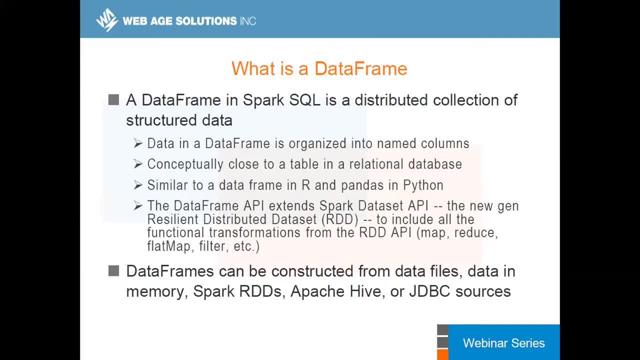 FlatMap Filter and a variety of others using pair RDD and very esoteric topics which we're not talking about here, but they're there, meaning if you have exhausted all your venues to extract data in the most efficient way. 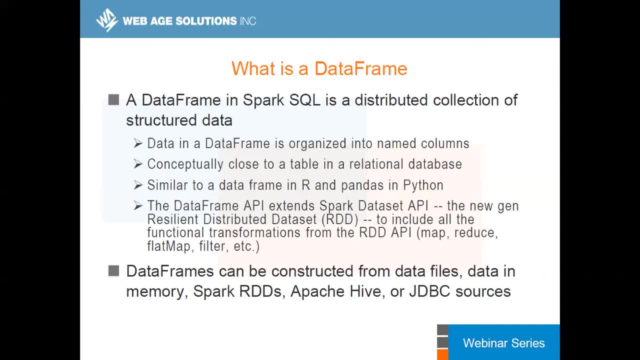 you can always fall back. There is a backdoor in the data frame to get through access. It's not actually a backdoor. It shouldn't be like that. I don't want to duplicate RDD. It's still there. It's just a matter of getting that last resort. 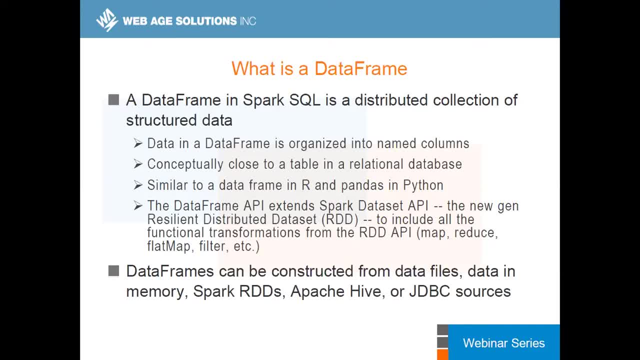 kind of plan B to use And it gives you a way to expand your tool set. So data frames. normally you construct it when you load the data from any of the supported data sources. You can construct it from data sitting in memory of those machines. 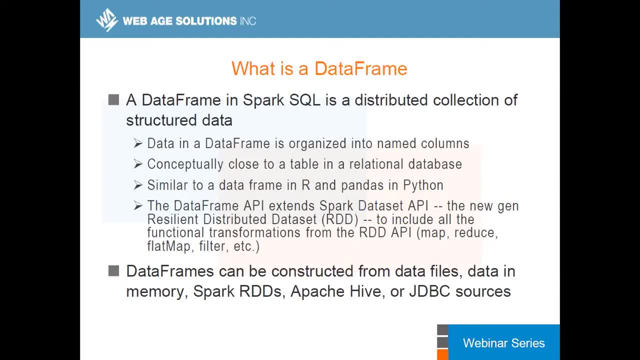 Spark RDDs is another source. You can read meta store of Apache Hive if you run Spark alongside with Hive on Hadoop and the GDBC sources. So you get the data from a database and you wrap it up in a data frame. Essentially you get yourself a very nice data frame. 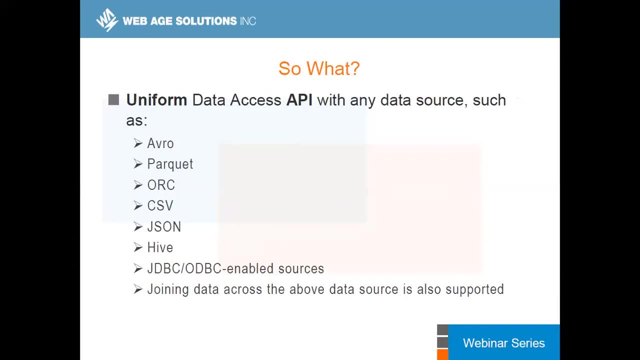 So the question would be: so what? Probably it's time, I'm not interested. It looks like it's just another kind of technology I have to learn. but what's happening is, the dynamic is now that people are trying to experiment and probably save some bucks on the licensing. 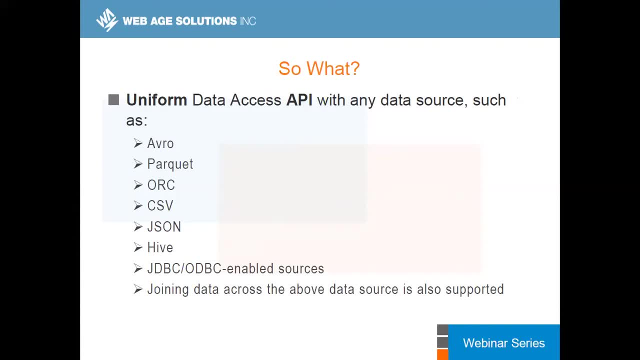 And Spark gives you a very viable, sustainable alternative to existing products in that space. Of course, Spark is gonna replace all those major databases that are currently used in production. They have their own set of use cases and they cannot be beat, be it online transactional processing, 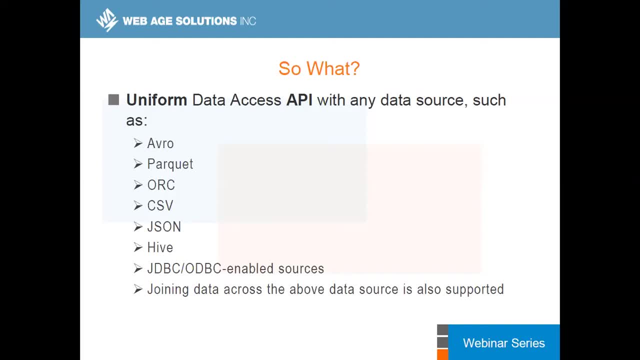 or very efficient clearing, But at the same time I guess that's a new wave of technologies that is here. It's not hype, It's not. I mean, I'm not gonna sell it when no way associated with Databricks or in other company AWS. 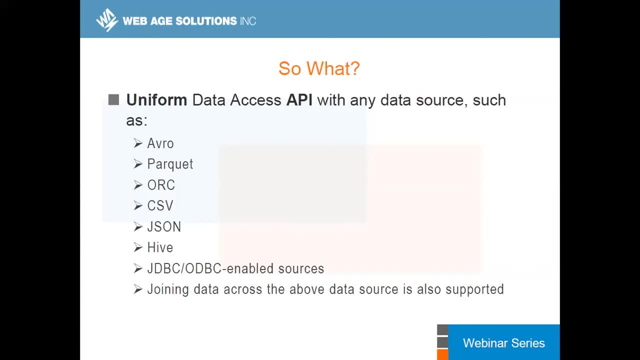 We just want to enable you, to give you the right tool for the right job. So, as Marshall McLuhan said- and I used his quote- we pretty much live in the age of anxiety. So we go to kind of a bronze age and we just slowly, we're slowly progressing. 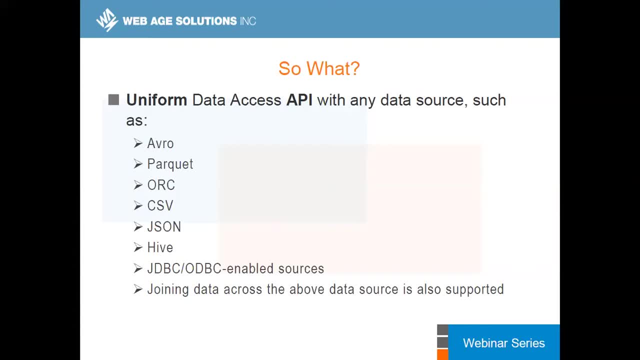 and now it's the age of anxiety because we are not using the right tools for today's jobs. We are still thinking in terms of old categories, old concepts, concepts and ideas, using all tools, um, so uniform api. so i mentioned that, i'm going to reiterate it. 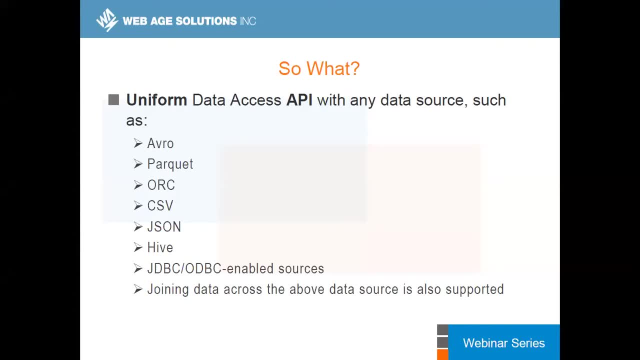 because that's what really uh done well. um, in spark you can also join data. so you pull out data from gdbc database and you can join with data uh frame uh built from, say, in memory so you can perform probably a very good fraud analysis uh system so you get the data in real time. you do. 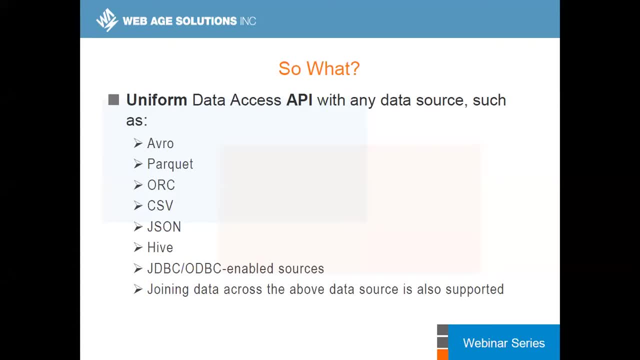 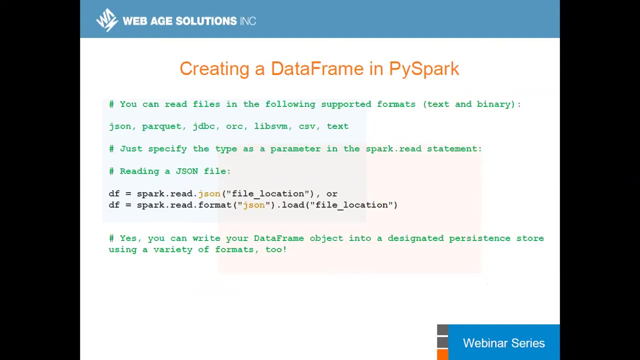 the batching, you extract the data and you run this batch across a particular time horizon, you get the insights and it can be done in almost near real time. so here's a couple of examples. so, um, it's um more of kind of a technical presentation, but at the same time i would 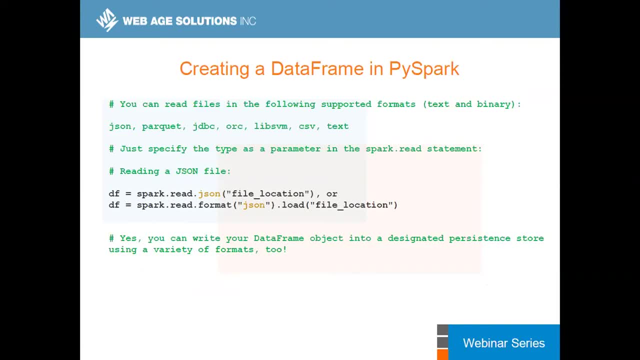 expect that you would see what is behind it, right? so all those um, kind of syntax, uh, things, so the statements, they just tell you the story that pretty much when you execute this line, we are using pi, spark, python on spark. it gives you a way to load the data in a specific format. uh, there are also 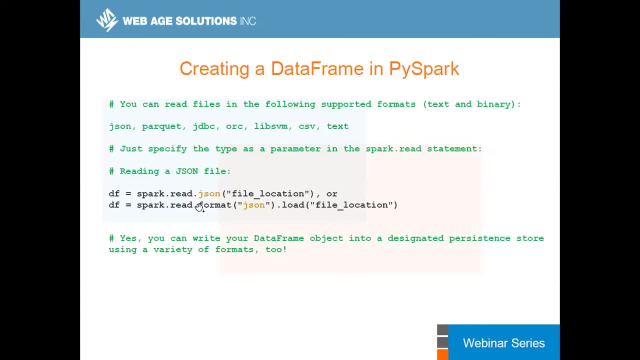 methods for uh, orc, um, the machine learning, lib, svm, format, parquet and what's not. there are two types of syntax. you can find one as uh. the read class exposes a bunch of methods which has uh, specific uh, for any of the supported file formats. you can also use another um method called format, which takes 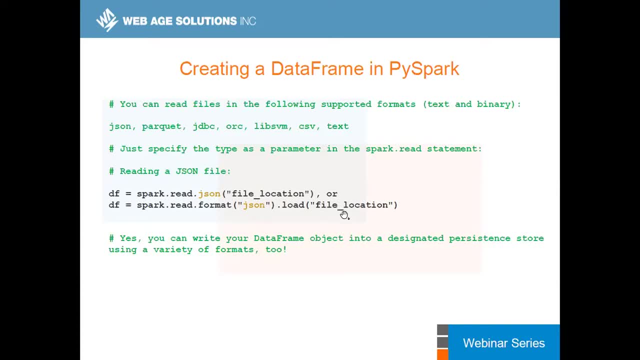 that type as a literal and you load the file from any of the supported storage types and usually people use hdfs because that's where spark plays really very nice. right and um, that's it, and on the left you've got data frame. this is python, if you're not familiar. 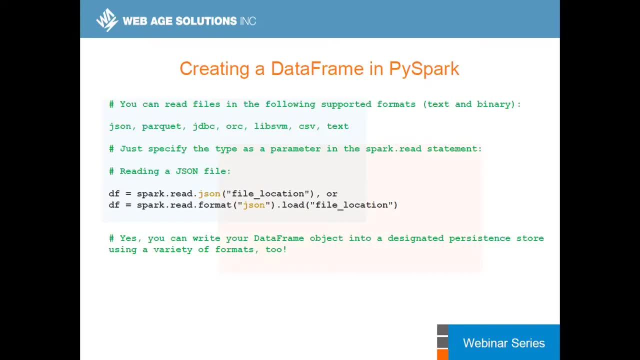 with python. i'll just quickly kind of give you a sense of what would it, what it does. so data frame is not qualified. it's not defined in any way as a data frame using any of the statically typed language. uh, things would be. So the statement on the right hand side will generate an object and Python will. 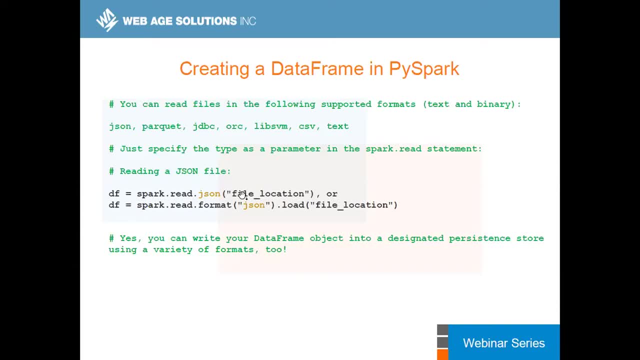 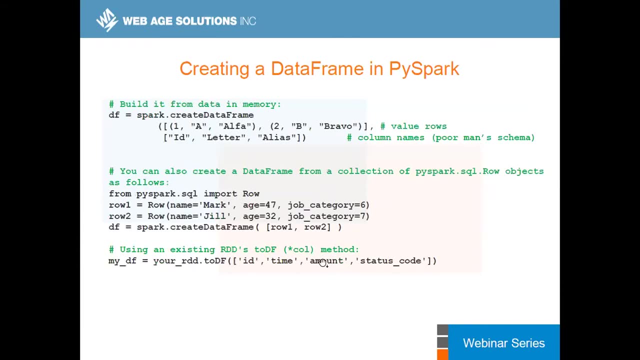 identify it as being of type DataFrame And then DataFrame will give you the API which we are going to take a look at in a moment. So we are just continuing with ways to create DataFrame. right, So you can create a DataFrame from data in. 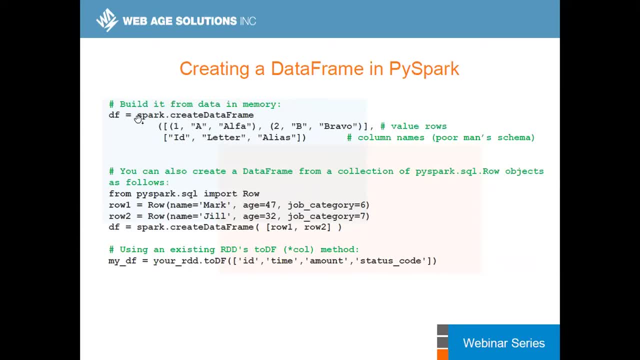 memory. Spark is a Spark context. it's a session object- pretty much just gives you access to a breadth of kind of wide range of methods and properties attributes that allow you to manipulate data very efficiently. So what we're doing here- maybe I will just quickly annotate it- I'll use red, So we create a. 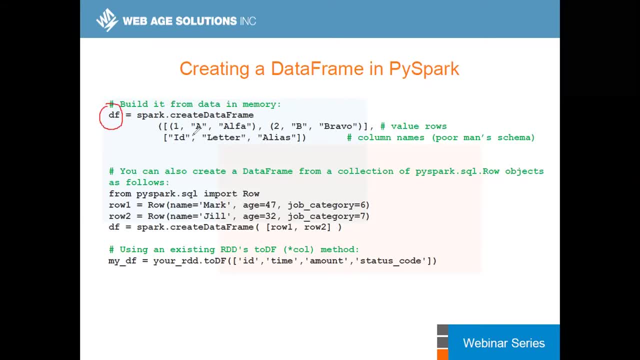 DataFrame on the left, right and what happens here- Create DataFrame very nice- speaks for itself. First we create value rows. it can be for lookup tables. you can create really data that you can fetch real time, let's say from database. we use arrays, so those square brackets- 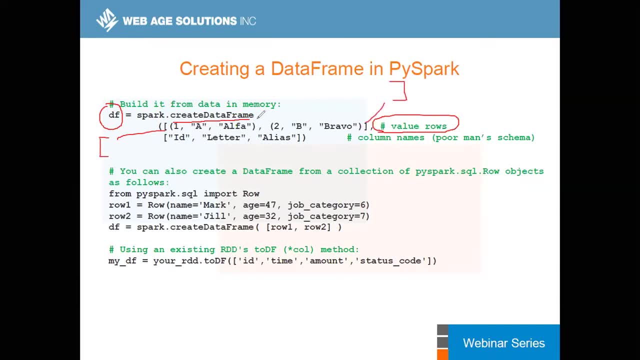 indicate that we are creating an array and python uses the concept of tuples, so those tuples around brackets essentially allow you create records. those are unmutable representation of your data which have columns, fields. right, we've got three fields, as we see, and in order to associate that value records with the with some sort of a simple schema, 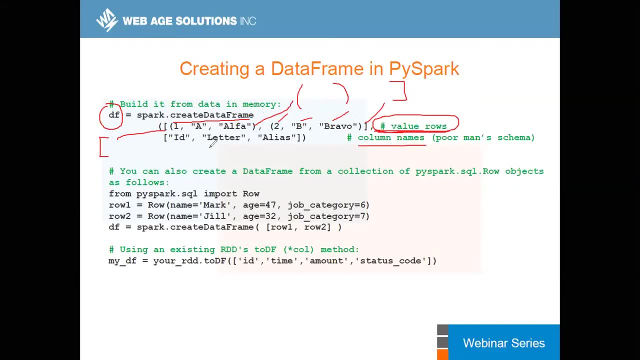 we would assign column names, okay, so we'll have every field from the tuple associated with the column. so pretty much you become someone who creates data frame on the fly. so that's also you can have a more low level where to create the data you would use. 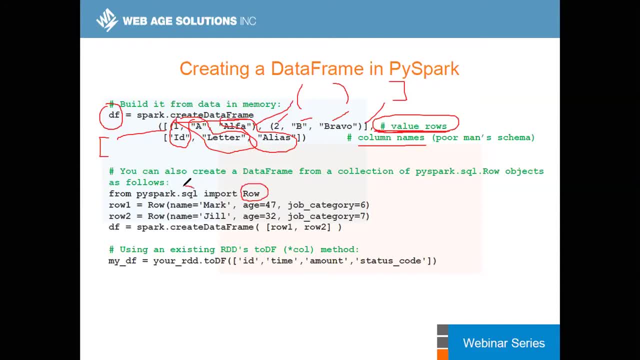 the raw objects that you would export from the sql module and then you would create all those objects and at this point in time you have very nice schema because things would be easier, because system would identify that now pretty much we've got everything associated. so on the left we've got. 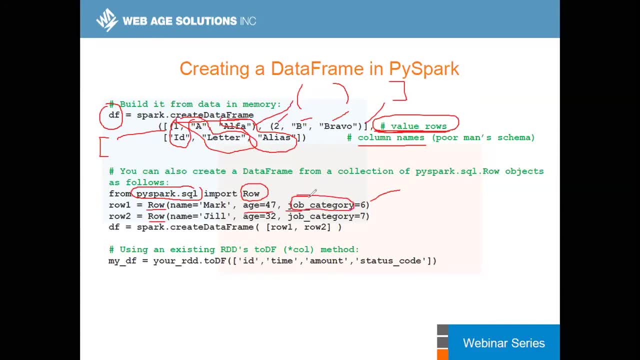 the most limited um, but you can also create a very small number of fields which give you a much bigger deal, right? how do you describe a single code on each one of them in place? so that's kind of what we're looking over, and some of you can even 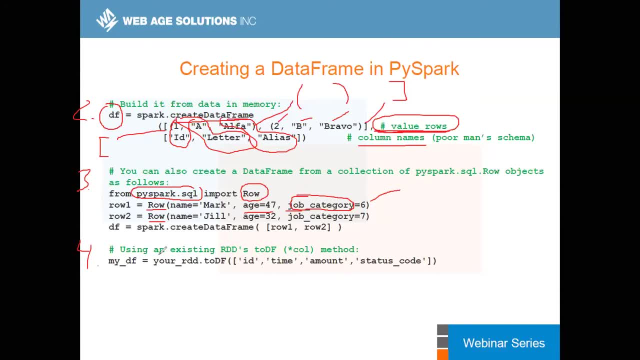 do that so you can use the schema mockup. at least you can use the schema mockup for every one of them. how can I get to that SPL? You need to do this step, You need to go through that And I pretty much, I guess, show you how to quickly. 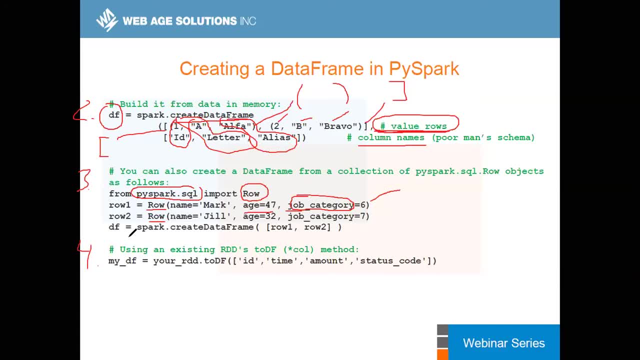 start applying your knowledge in production without delaying and putting it to kind of a forget it button bucket. So let's say you've got an RDD that you somehow generate. You might have read it from any of the other sources, let's say from HDFS. 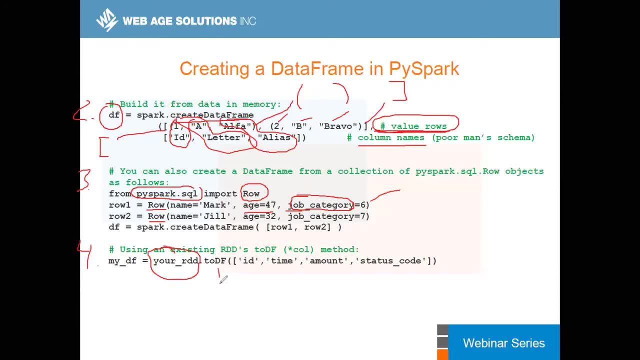 It has been probably serialized in some way And there is a backdoor that I mentioned, 2DF. So essentially you've got yourself RDD and it allows you to convert the records stored in the raw format in RDD. RDD, pretty much is just the assembly type of thing. 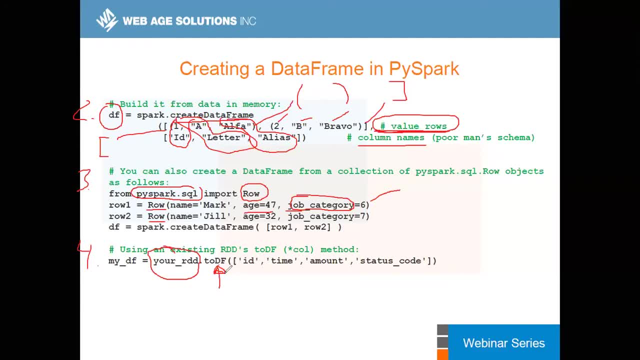 Low level, very efficient with lineage. all the infrastructure things are there, But data frames are nicer. They are more user developer friendly. So what you do here? you just take all the fields from the every row in your RDD and you assign column names. 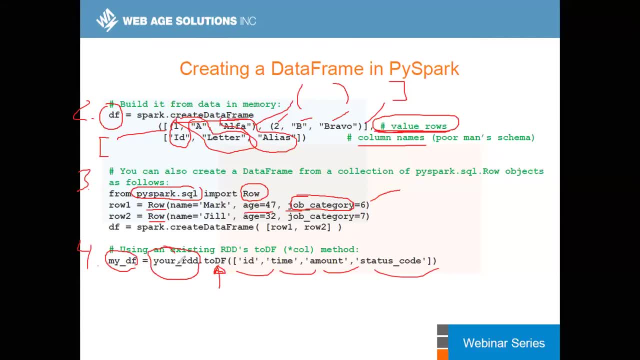 So essentially, your data frame would be the original RDD, which has been decorated with columns and some additional information. Again, if you have any questions, let me know. put your questions. Let me know if you have any questions in the chat window. 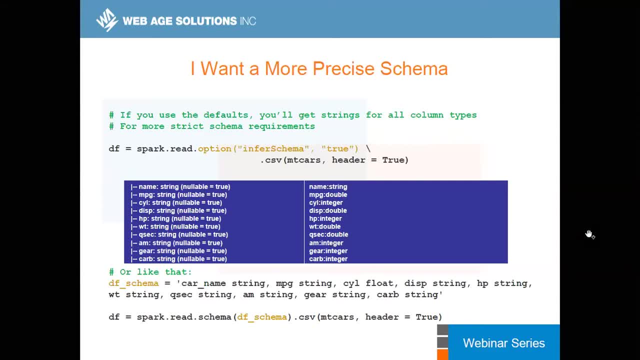 So the first question that people- maybe the second question that people- start asking: how can I create a data frame which caters for some specific requirements, data requirements in the data set, And usually it comes with accurate schema which, by default. 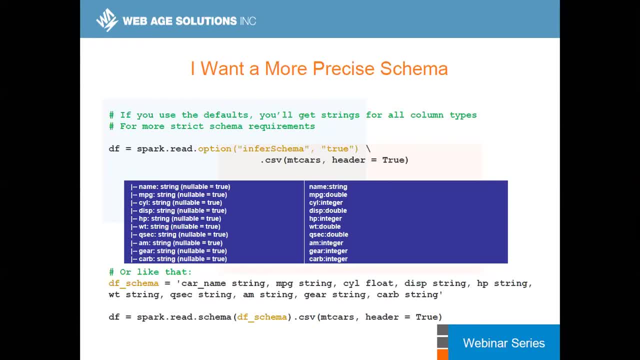 when you start creating data frames, everything is treated as array of characters. It's just a string, right, And in many cases it's not what people want. Of course, you can convert the string into double value or an integer, but that's not the case. 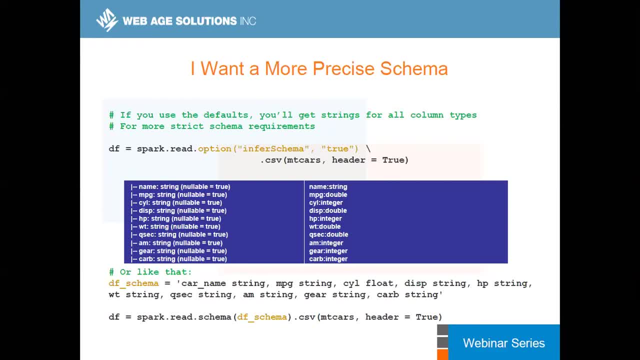 How we can do it in one kind of a fell swoop. We just start doing it when we read the data from a particular source And we would like to have very accurate schema because we know a priori or otherwise, that's what we want. 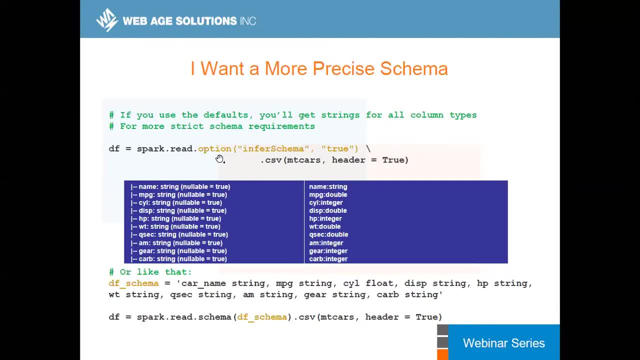 So, if you don't do, if you just read the JSON or the CSV file on the left hand side, you will see that everything would be string But NTCARS. it's a small data set which is very popular with our folks. 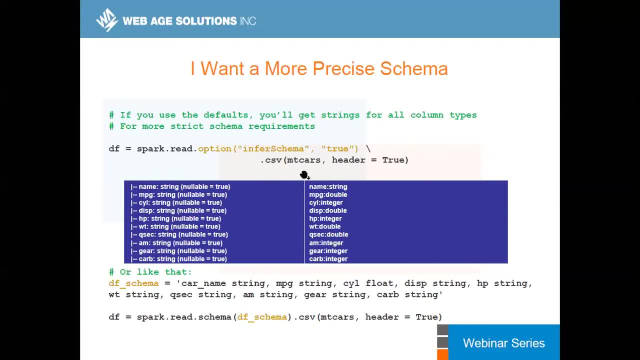 And just shows you that a little bit of the main specific object. Everyone understands in one way or another about cars, about engines, number of cylinders, miles per gallon, displacement of engine, horsepower and things like that. Right, So if you specify the options that you would like, 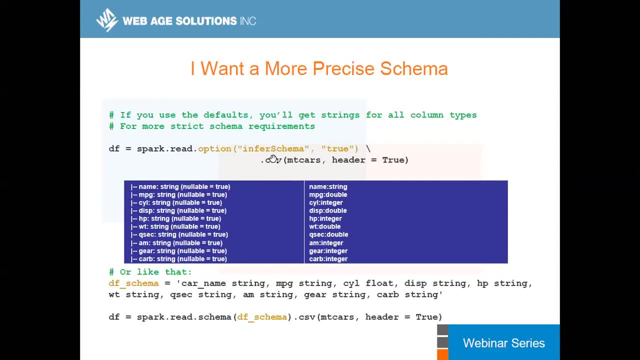 to infer schema. what Python, or more specifically, the infrastructure of the Spark SQL module, would parse the data. it will apply some heuristics and it will derive that understanding that it would be better off to use miles per gallon as double right. It's just because there would be a decimal point. 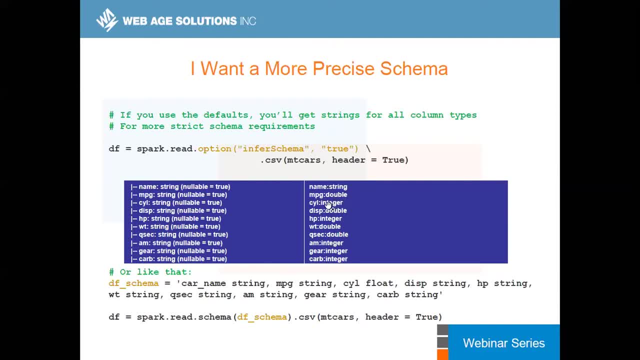 in that column Cylinders. it's an integer number, it's whole number. more decimal points should be used. As you see, our system. it's quite simple, right? It's very simple. It's quite intelligent in getting those insights. 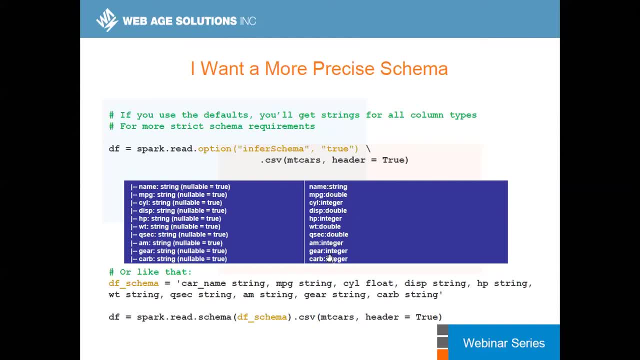 and you get yourself a nicely organized schema so that you can have a better performance and a nicer API Right. Also, you can specify schema on the fly. When you read the data, you just create that string which has kind of touch to the value elements: card name and string. 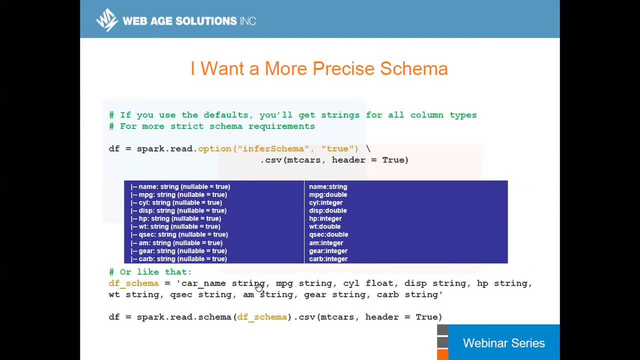 essentially it's a string, but it's just a. it's kind of a key value pair. It's very nice way. What's good about Python is I don't really think that they would look kind of stupid once it does things like as simple as that. 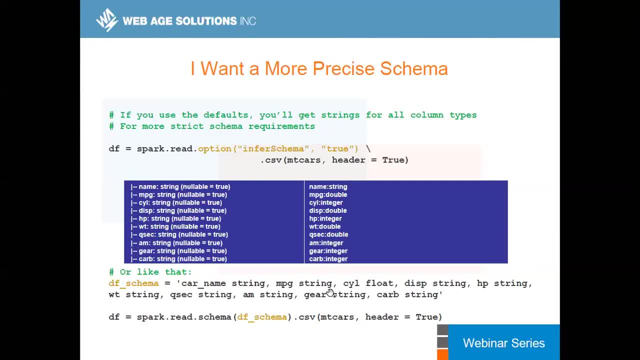 More enterprise minded people, folks like from Java. they would probably create an XML or VC data release schema or something else, So the schema would define the schema and data frame, And it can go on and on. I worked in enterprise space for quite a long time. 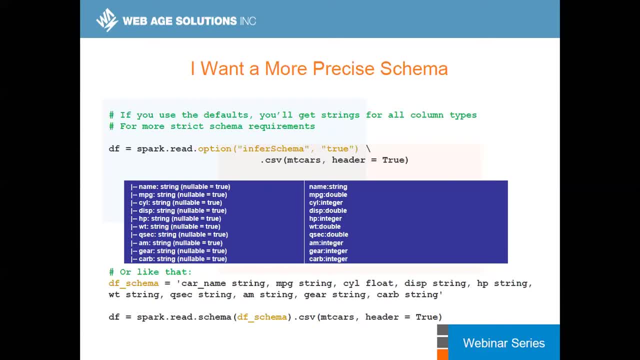 I'm a certified enterprise job architect and I know how to make it look very formidable, very serious kind of, so that you can kind of puff your cheeks and just go as if it's just you solve the world hunger problem. But Python is much more, I would say. 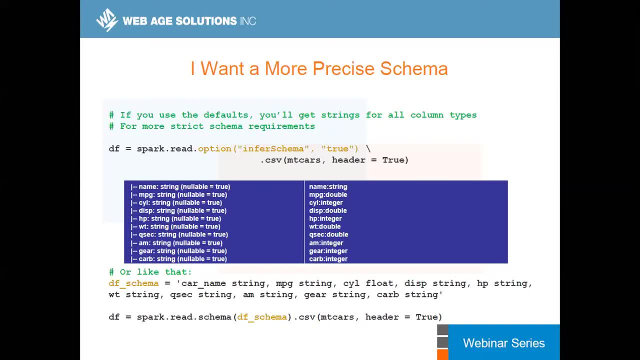 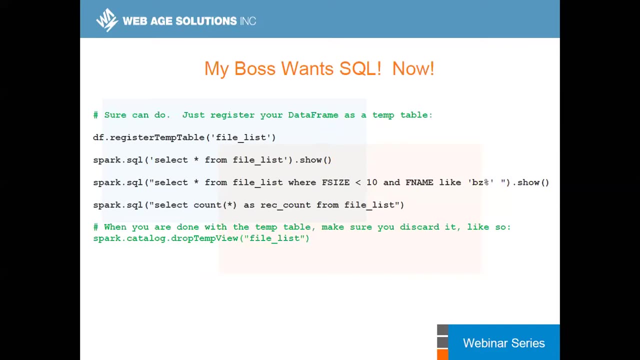 it's much more agile. That's what I guess most appropriate adjective that you can use in this context. And then header is true. it speaks for itself. So now you've been talking about this Spark SQL, So now, where is it? 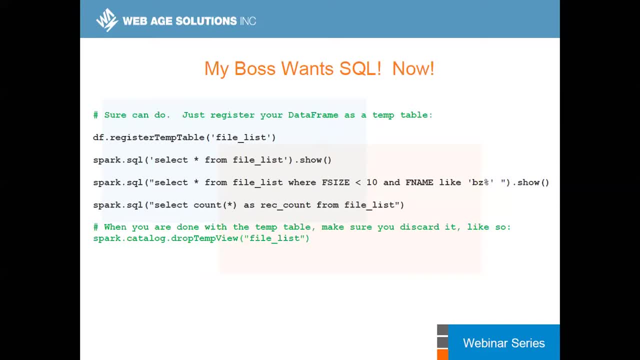 And that's what it is Essentially first thing that we need to do. let's say you created data frame in one way or another and then you can do the following things: You need to register it as a temporary table. Spark or Spark SQL will create that infrastructure. 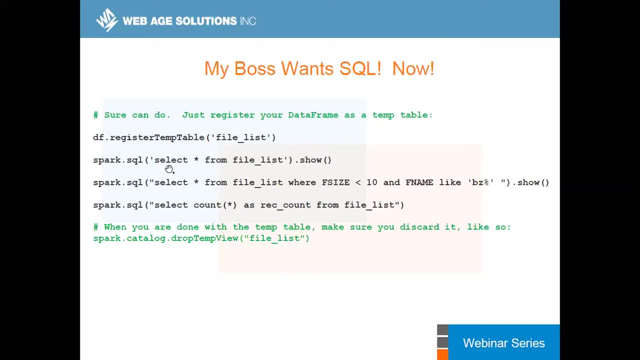 for you to start converting that embedded SQL that we talked about. SQL is a method of the Spark session. It's kind of a Spark context object which exposes SQL, but you can only run this SQL against something that is known as a temporary table. 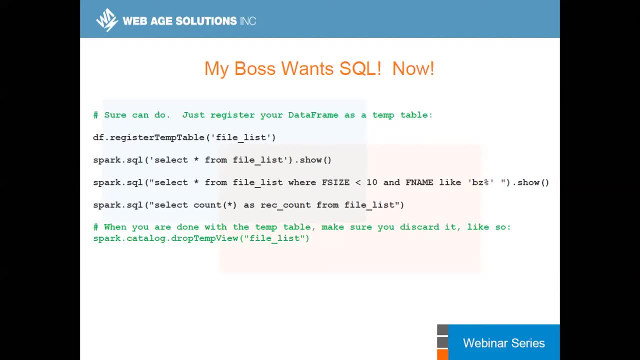 So let me just quickly walk you through how to do that. So first we create a data frame, right, We register it, So this is sort of a logical name which would be used by some optimization mechanisms, used like catalyst, And then we use SQL methods to issue embedded SQL. 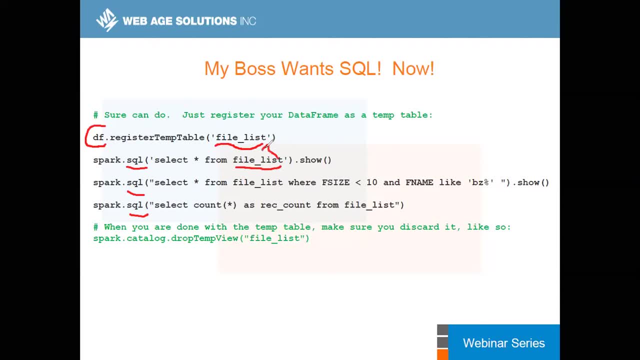 against the table That's. it Show means just brings data and display it as a driver process. So you can have quite elaborate SQL. You can do grouping, you can do filtering, you can do some regular expressions, You can do counting, averaging. 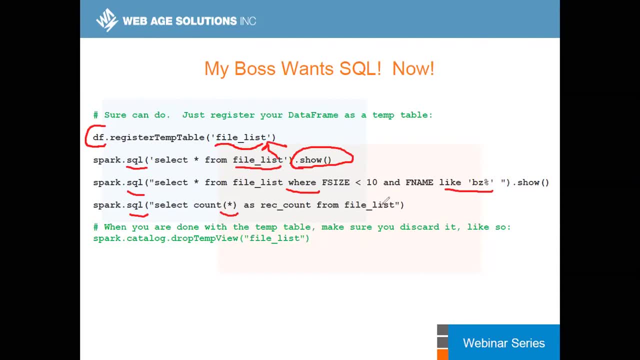 and having these else to support it. So that's pretty much what you can do. It's at this point in time you can say it's always advanced. It's advanced because you now are able to run this query against potentially hundreds of machines. 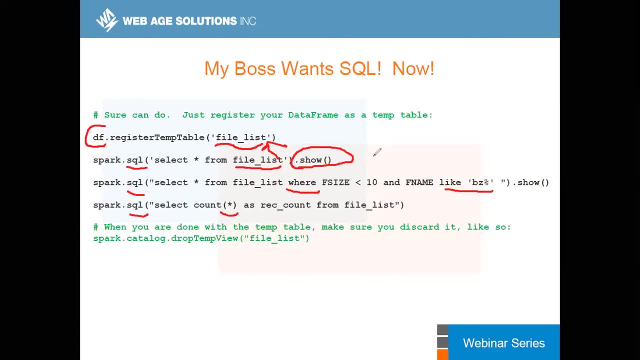 So that's the way the Muslims account. It's not coming from select. There will be a couple of points later on, but that's the point. So you use pretty much SQL which runs in a distributed manner. Those people who come from Apache high background. 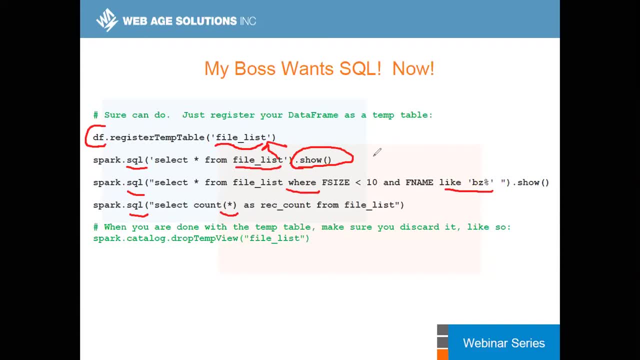 they would say: we can do it in Apache highway- and they will be right- But not just taking advantage of the optimized by default high runs on the MapReduce engine. Of course you can switch to Apache TAS or you can use Apache Spark engine. 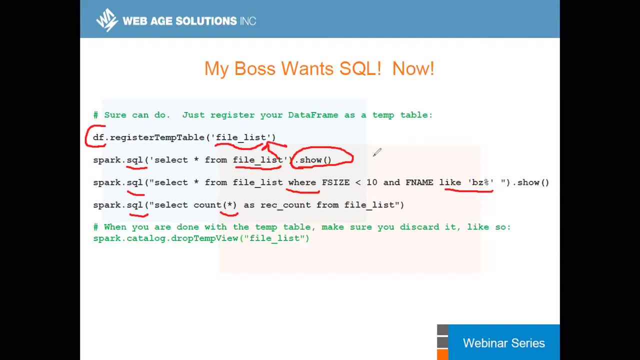 but it would require some experimentation and setting doing the things right. Here you've got SQL just embedded right. Don't forget to drop it Because, again, when you start experimenting, many people will get frustrated because at a certain point in time, 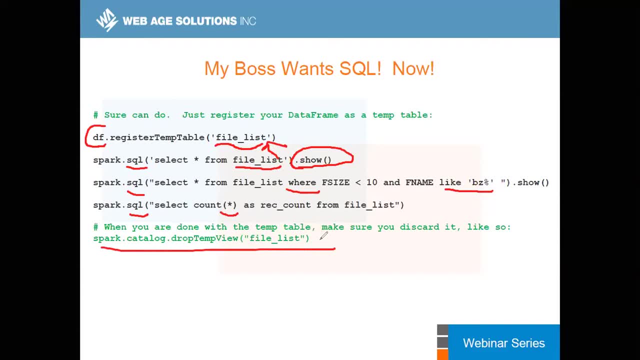 you'll start getting out of memory exceptions and other ugly kind of manifestations of the fact that you haven't done a good kind of thinking, You haven't cleaned your memory from. those objects wouldn't be discarded automatically. They would be sitting there, consuming potentially. 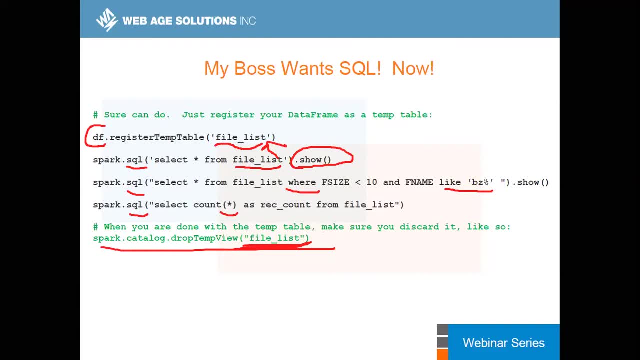 a lot of space In terms of presentation. I believe you should have received a link to that PDF file. I don't think that I would be able to do it right now. Let me send an email to our back office people. Just give me a second. 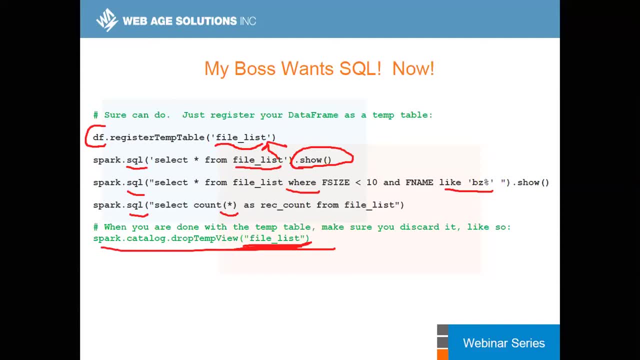 Yeah, I don't see that I would be able to share that with you. Just give me a second. Just give me a second. Yeah, it's a really good idea. I'll send you a link to it. I'm not sure if you'll be able to see it. 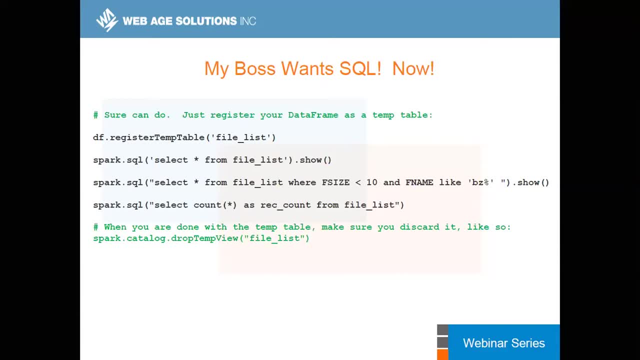 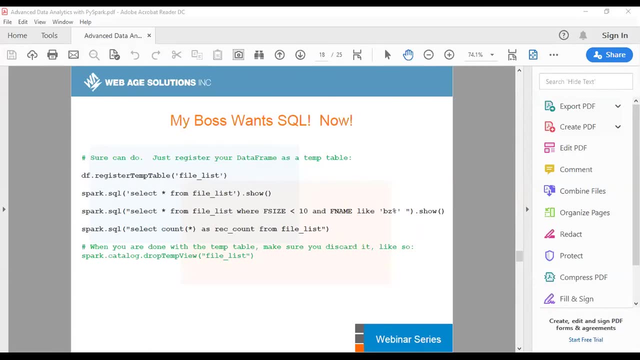 I think I will. Let's see if we can. Yeah, I'll send you a link to it. I can Let me see here. No problem, I'm going to put this in our. this is a pretty nice browser, Go ahead. 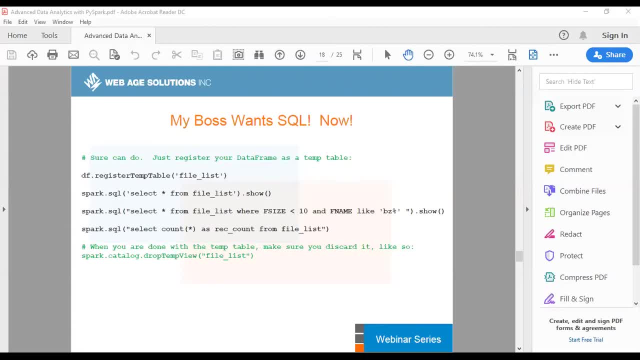 That is your home. I don't want to worry about it Because I have so many other things. I haven't done it yet. That's fine, Thank you. Okay, guys. sorry for this delay, I guess. Yeah, I haven't been able to share. 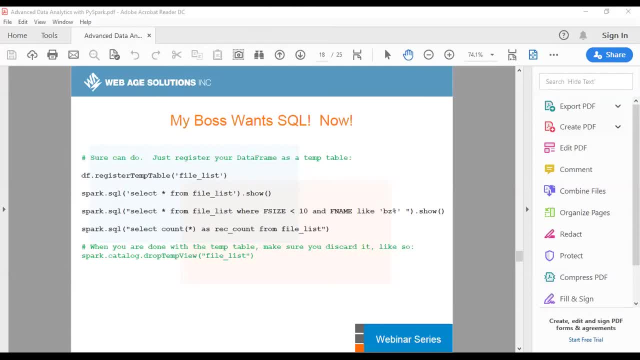 Usually when you use other tools, you would probably be able to see a much richer API where you would be able to upload files so that people can download. But I've got the slides. I don't have any problem. It's in public domain. 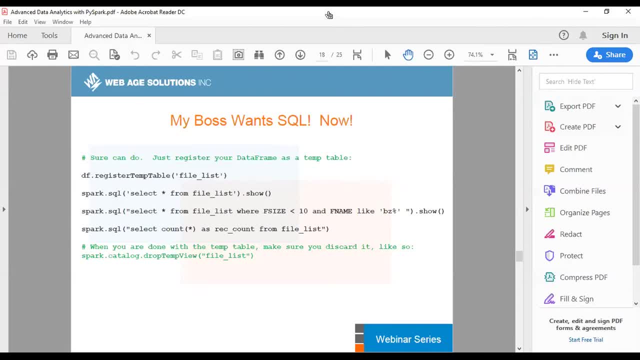 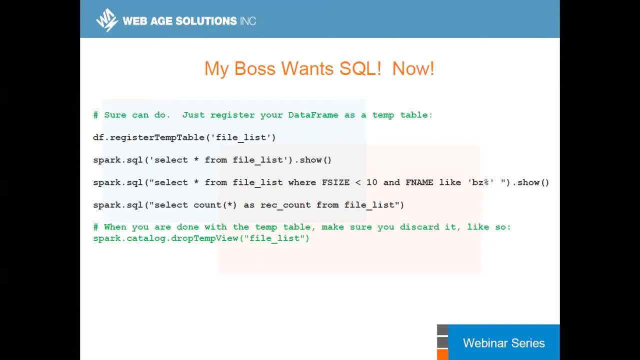 So let's continue. So that's SQL right. It's just a nice well-rounded And you know SQL right As long as you know the field names. How would you know the field names? So there's a way for you to dump the scheme of DataFrame. 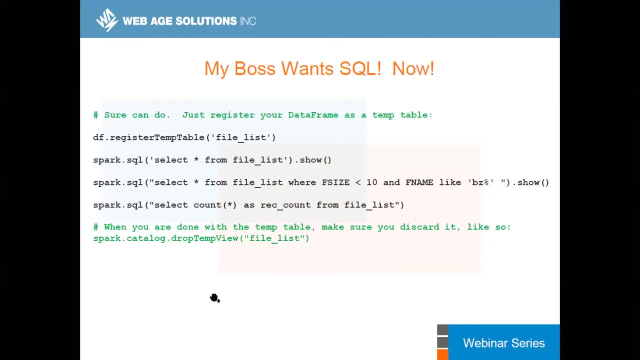 like dev print schema, or essentially you define schema here. So that would be the column names, And column names would be used in that SQL that you run here. Okay, so it looks like we're good here, So now right. 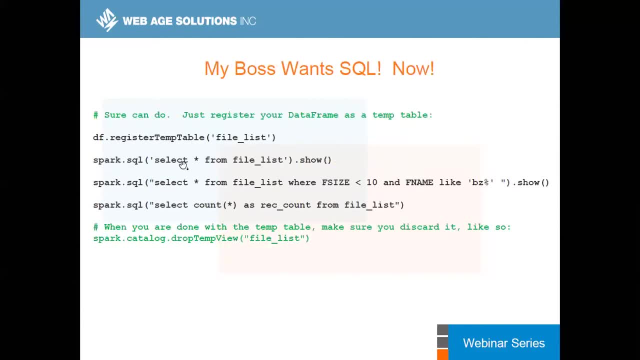 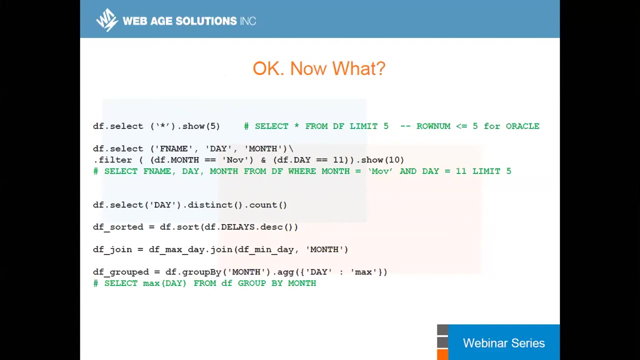 So, in addition to SQL that you would be probably very close, dear and near to many of business analysts, You can also kind of emulate SQL by using: Yeah, it looks like. yeah, Sorry, I was looking at the chat. 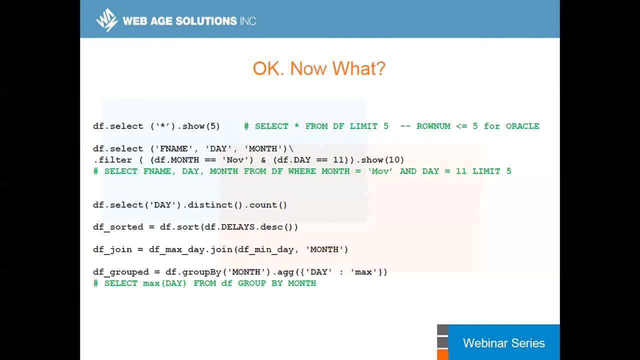 but it looks like some people are using the questions and answers panel. Okay, good. So the question is: what's the difference between temp table and temp view? So with view, I don't know exactly, because I only use temp table. 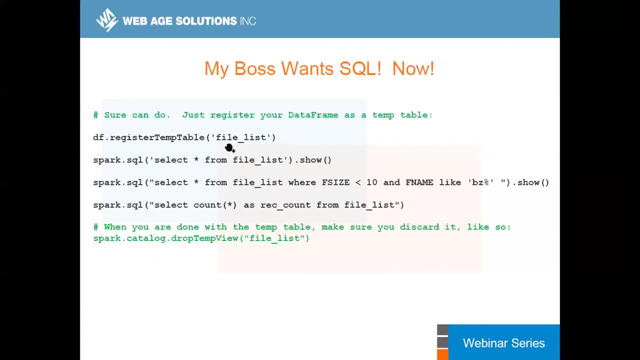 A temp table would allow you to use data right. Temp view would probably allow you to only use data for reading right If that is supported. I haven't explored that capability. And another question is: do you know how Spark handles count distinct with group data? 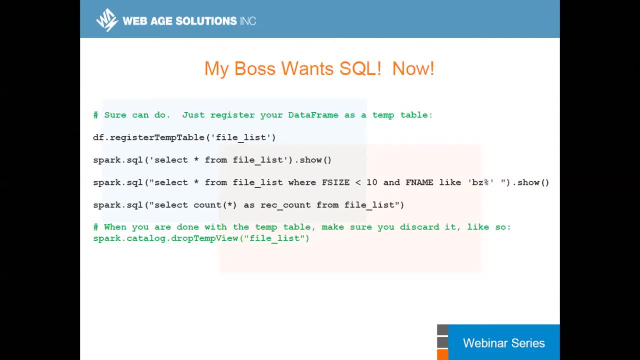 Yeah, sure, Yeah, I am a fan of count distinct with group by. It's not easily parallelizable in general, as intermediate results from each node needs to be collected in one For the final number of unique values. So when you perform distinct, 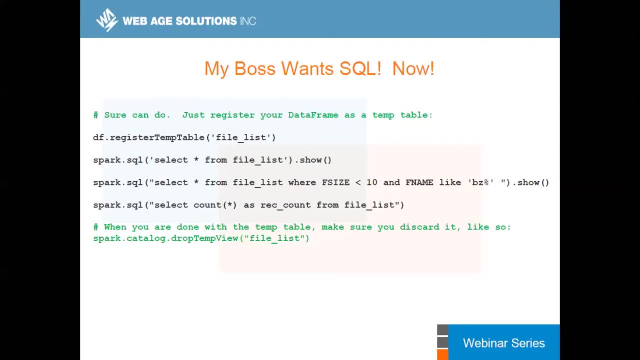 distinct essentially can be run. You can pretty much break your count distinct group by into multiple staged slides and so on, staged scripts, right, So you can help spark a little bit at this point. So you would probably perform like finding distinct values first. 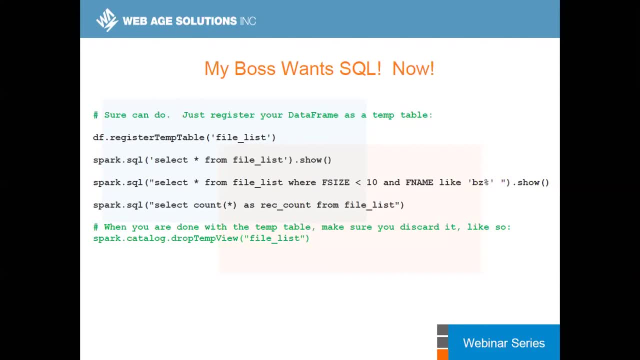 and then you would apply a group by against that. So it's possible in some cases, but you're right, In terms of parallelizing queries on cluster machines, it's not always possible because things would be shuffling, sending across And one kind of a big item. 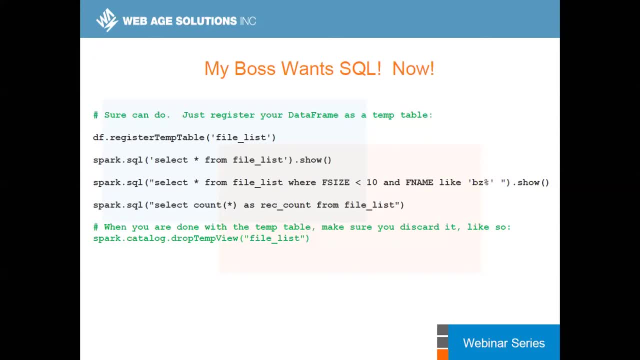 big ticket item. solution is to use lookup tables, which are broadcast variables. So what you can do, you essentially can have probably some pre-built, maybe artifacts that would allow you to simplify lookups And broadcast variables. they use UDP, It's kind of. 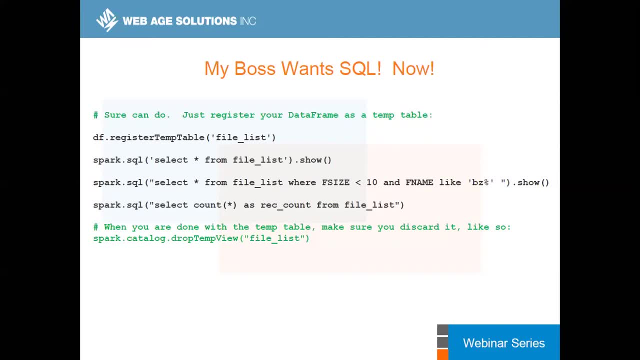 that's ubiquitous protocol which allows you to efficiently share the broadcast variables- kind of a lookup tables- across the cluster And then on every process, on every executed process, you would use of the broadcast variable to look up and select the values right. 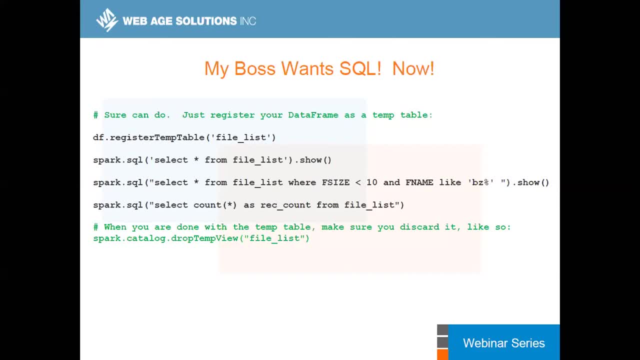 And it can be parallelized, And then the aggregation kind of when you need to pull the data down back to the driver process. it would take kind of much less. I guess heat- It will be less painful, right. 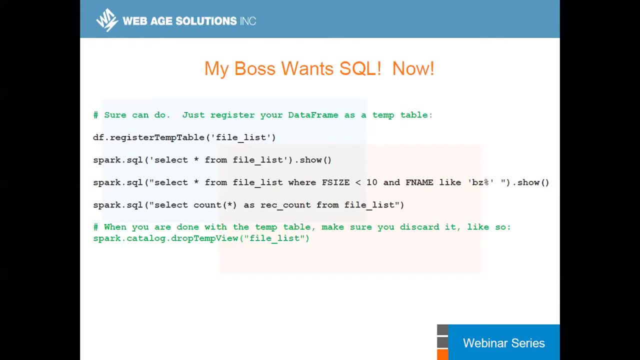 So it's a big topic, right, It's kind of a big big thing, but definitely the solution would be: don't try to put as much in just one query, right? So it would be suboptimal And that's what kind of confuses people. 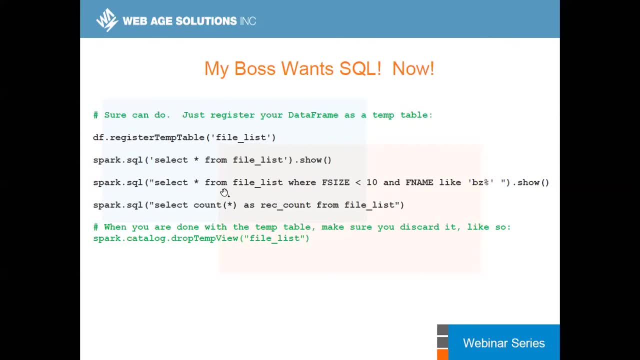 Yes, you've got Celiac. but even though if you have it, it doesn't mean that you have to use it in this way. Now, same applies with using functional programs. It was MapReduce. People start using that kind of a chaining apparatus. 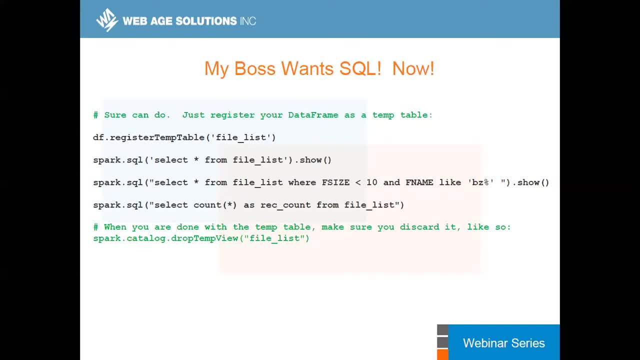 using dot notation and it goes on and on and on until people get out of memory exception right And it just starts really frustrating people. So don't just try to avoid things, Just try to partition it and think about in terms of kind of how to process data piecemeal. 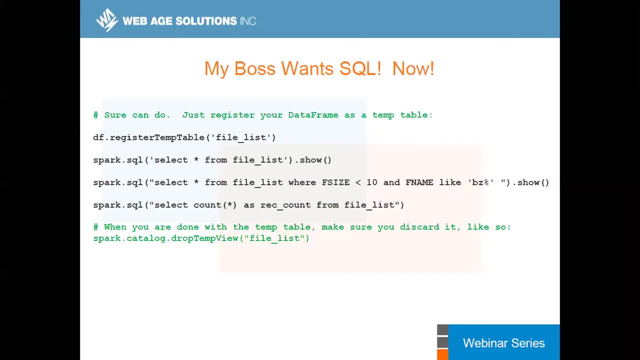 You probably would need to do reorientation of data but, having said that, it would be much more easier for you to do it using the DataFrame API or using Scala Python- just the functional programming as opposed to just one single SQL statement. 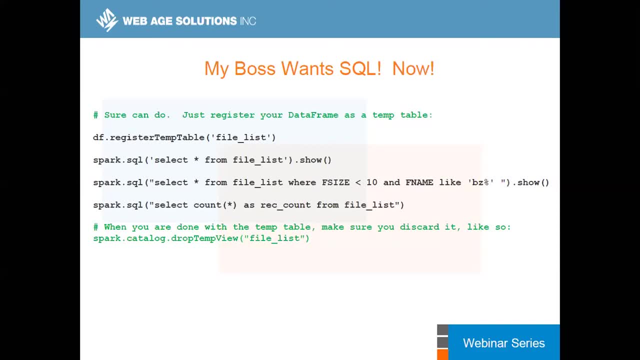 which we would use. Of course you can use PLSQL, TSQL, other systems which would allow you to do this partitioning, kind of piecemeal processing, but the programming API of Spark SQL is just lends itself to kind of a staged processing. 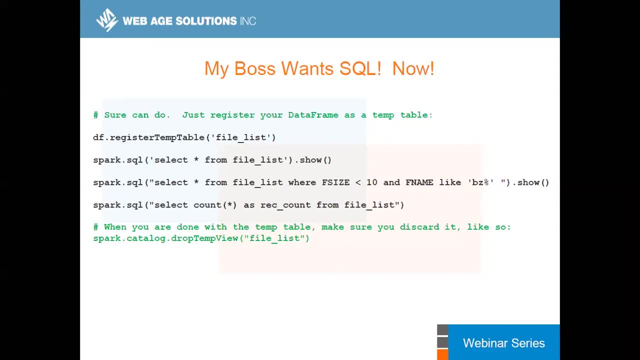 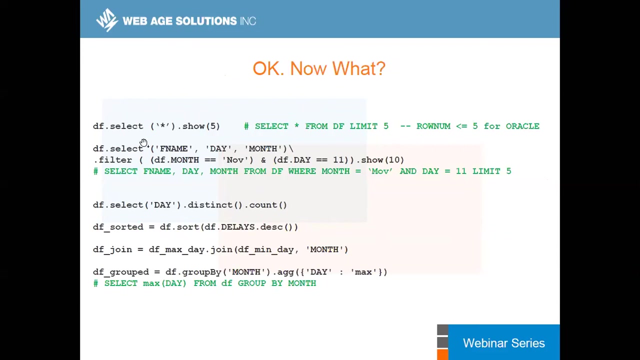 Hopefully then this answers your question. Okay, Right, Okay, so moving on. So we've got kind of the API that allows you to emulate the projection select projection statement. Right, So we've got a very nice way. 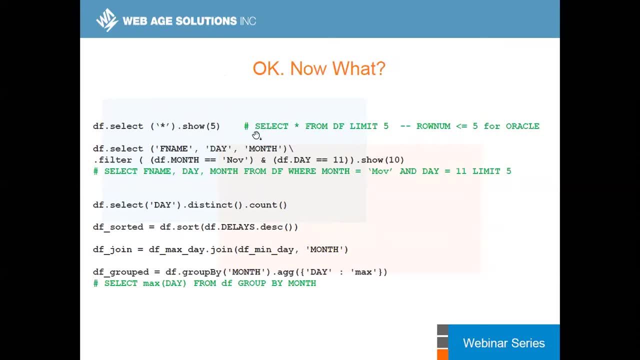 And, by the way, this slide just shows side-by-side the actual DataFrame Spark SQL API, alongside with the select SQL statements. So that's what you can do. I'm not going to read unless I see something that would require some clarification. Yeah, in some cases you can use the select. 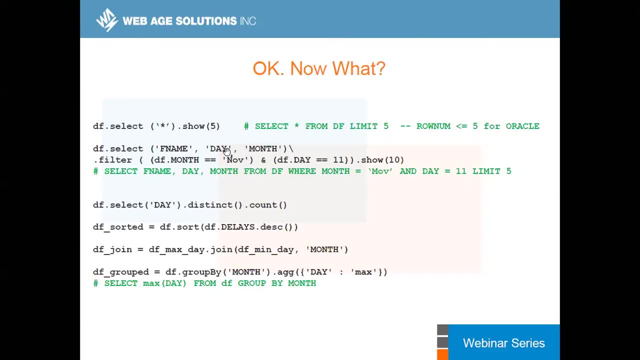 essentially just emulates the select, select, close projection So you can specify the names of columns but also what is supported. is that documentation and Spark, like Jupyter Notebook. it would allow you to use auto-completion So a system would keep, would cache the schema. 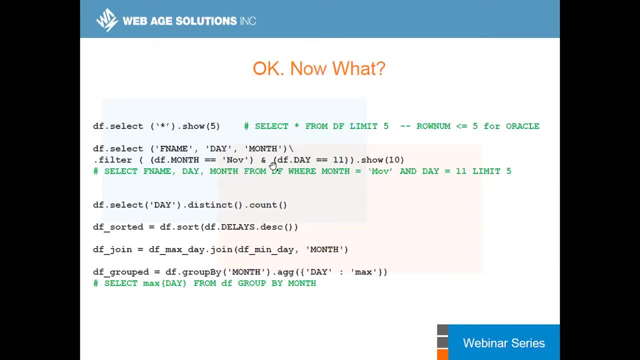 that is associated with DataFrame and you can use things like that. Okay, so field is started close. So you can do distinct, select distinct days, IP addresses, credit card numbers and those account right? So again probably back to the question of green with this. 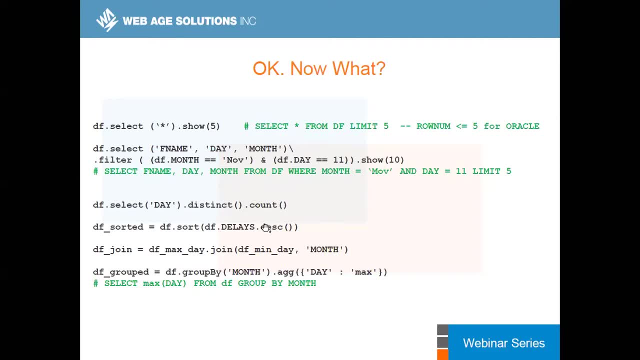 I guess you can play around with maybe DataFrame in this way: Yeah, grouping, So let's say you group days by months, or something like that. Let's say you group days by months, or something like that. Let's say you group dates by months, or something like that. 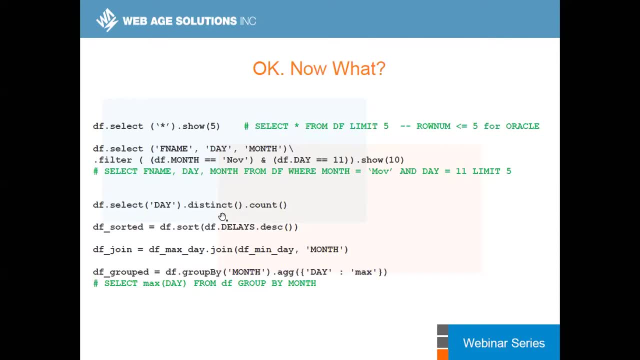 by months or something. So I guess somehow you can just start looking from this point And time, definitely timing all the processes, how long it takes user time, kernel time is important. So forcing data: it's similar to the forcing data in SQL. 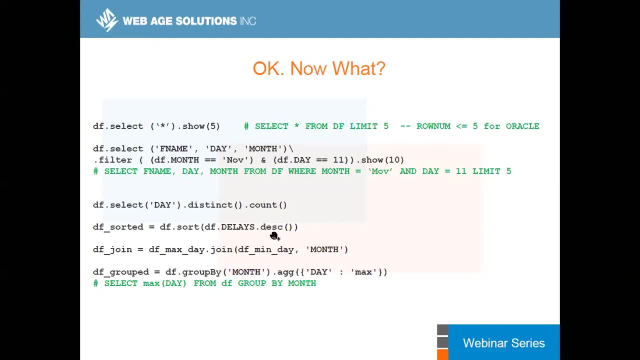 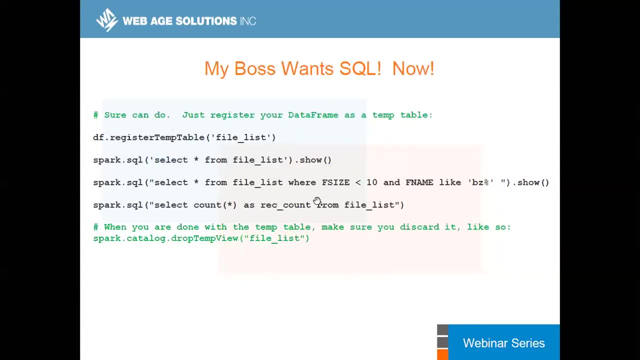 By default it goes in ascending mode. If you want to do descending by a particular column, you need to use that method. So it's a little bit different from what you would do with SQL. Of course, if you want to use SQL, you can use it here. 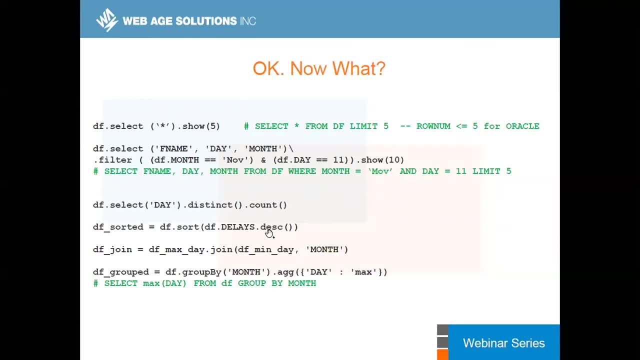 And here you would be dealing with only DataFrame type of API. You can also join tables, join DataFrames, And DataFrames should have that single month field or column that would allow you to join one DataFrame with another. The join DataFrames you can do left out, right out, join. 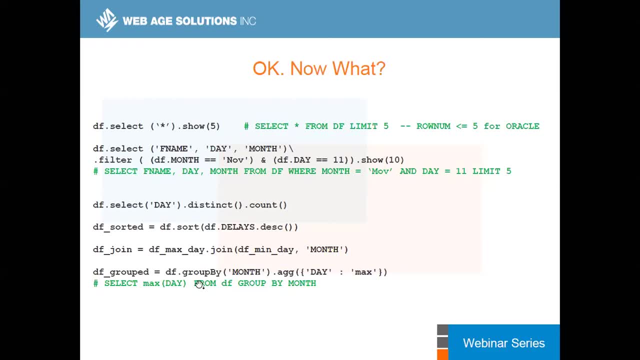 Here's a grouping operation. So the grouping would use the group by a method. but you can also, if you want to find aggregates within those groups, you can use that. You can use JSON type of syntax aggregation. It's a method which takes that stanza. 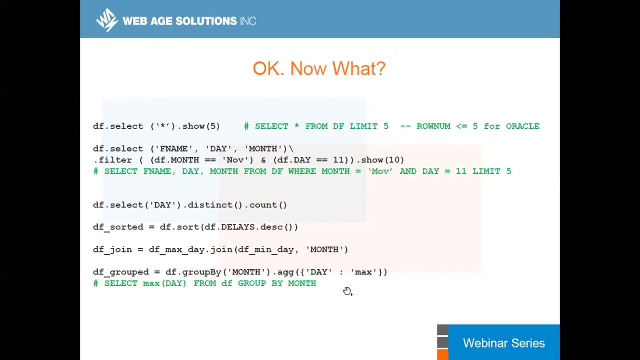 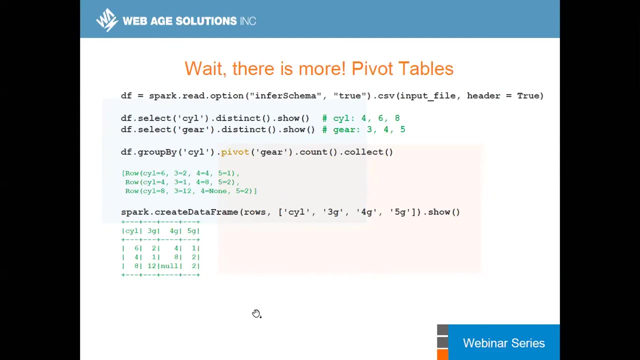 and it does aggregation of finding the maximum value for days which has been grouped by months. right, So that's what an equivalent SQL statement would look like. Okay, Pivot tables are supported, and this is just a brief, So that's what I guess. 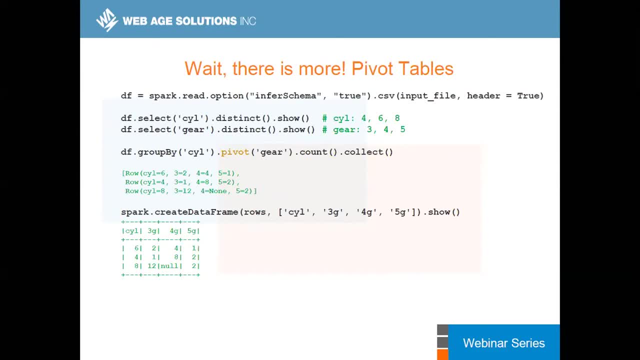 what is interesting about the DataFrame API: It's absolutely easy to just create the pivot table from any values that can be kind of treated as categorical values, as some sort of enumerated types, Like, for example, the authentic arc. it has two factors, factor variables, cylinder and gear. 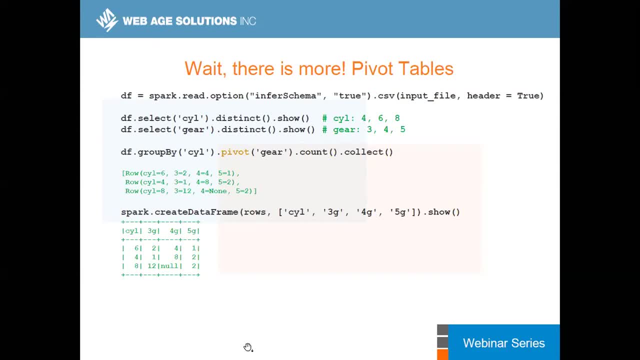 So there are three values for each, and that's how you create a pivot table. You do the grouping, So essentially, you designate the columns. that would act as kind of a row and the gear would provide the values. So there'll be three columns: three, four, five. 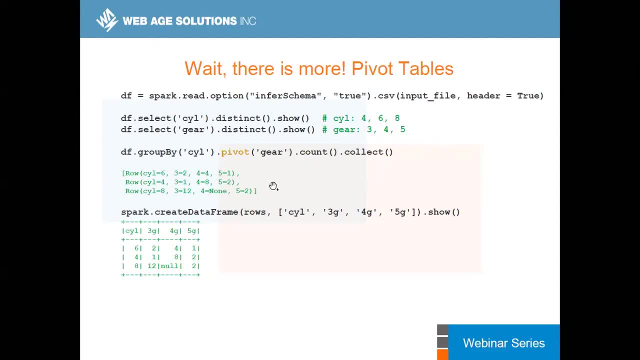 You perform counting of occurrences of records which would contain the intersection of cylinders and gears. So that's what would be the raw API output of that statement when you run it. Collection means that you bring the data in the driver memory right, And if you would like to visualize it, 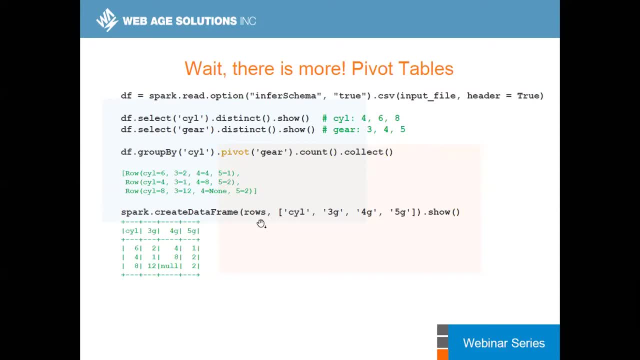 and have a nicer way to do this. that would be the way. So you specify the rows and the rows essentially returned by this statement, and you specify the columns, like loss would come from pivot and cylinder would comes from the cylinder value, And that would be a very nice aggregate value. 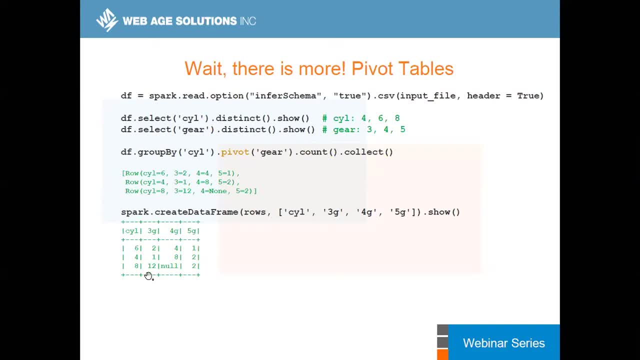 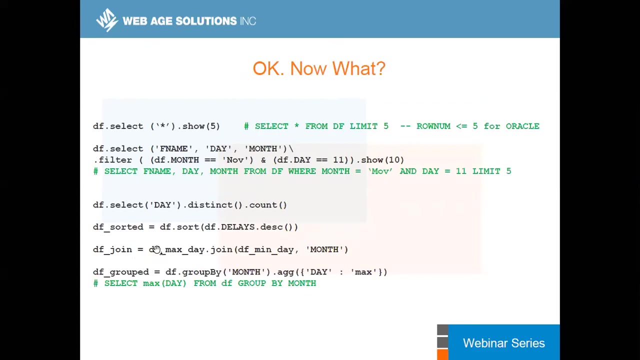 Mal means that there is no car with eight cylinders and four gears for manual. So there's a question created out of mail. Do you have in this example? Yes, those are kind of separate data frames which have some relation and the relation is expressed. 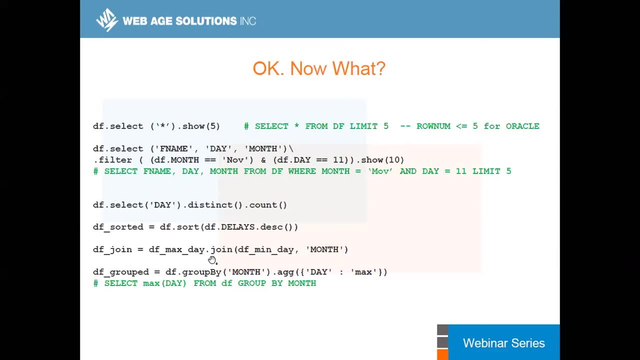 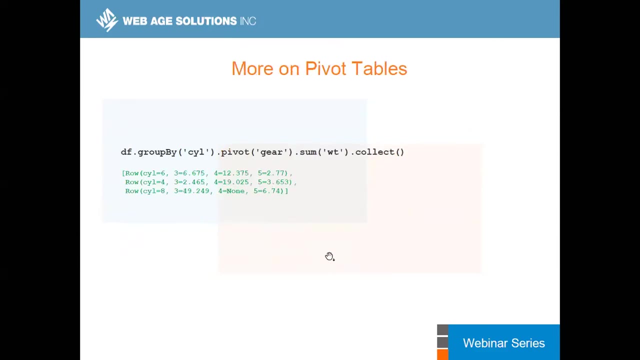 in the months and we just want to combine. So we potentially might get it from different sources, from different vendors, but they should have similar structure, sharing that month's goal. Hopefully I was able to answer right. That's it. more pivot tables. 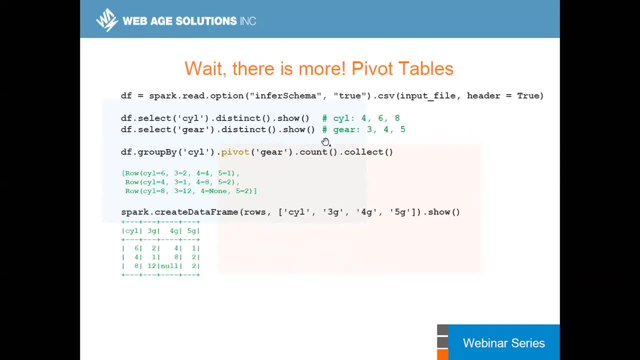 So this is kind of a more of a summary report. You get the data, you combine them quickly. That is a very powerful operation and you just wait right. It's good And, by the way, what you can do at this point in time. 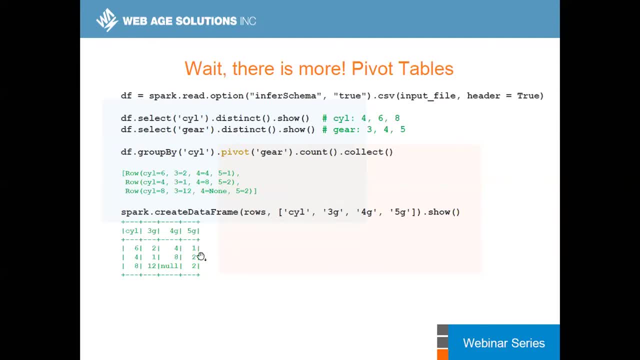 you can do some sort of a heat mapping. You can apply some labels of the visualization. You can build a bundles table. Unfortunately, as the client for this presentation doesn't allow us to give you a better idea, Give it at a good mountain of standing. 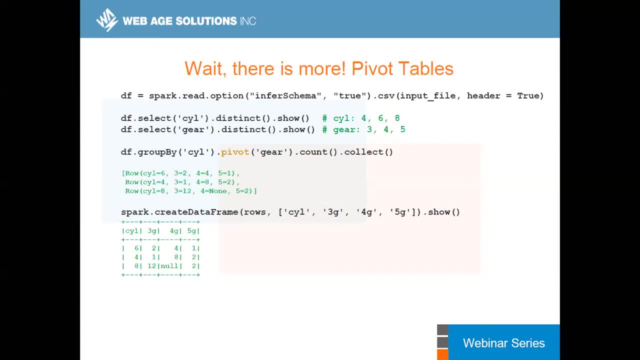 Done a better kind of a coverage of the material that we have, such as EDA in sporty data analysis using pandas, deboard and you can see, just to give a very nice executive type of summer. Also, you can do a more elaborate. 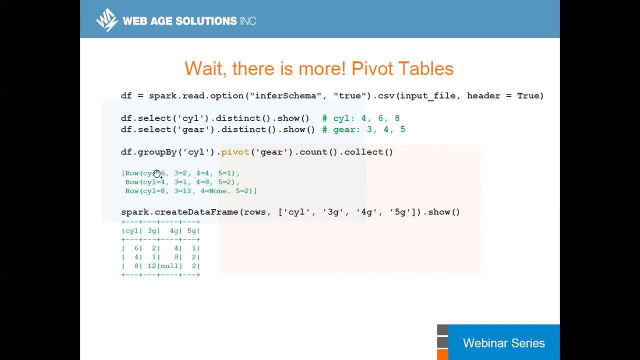 So here we use counts over the course number of machines which have those. if you would like to find some weight is I guess it's a weight of in pounds, or a car divided by one thousand. I don't remember exactly, but essentially what this operation does, it allows: 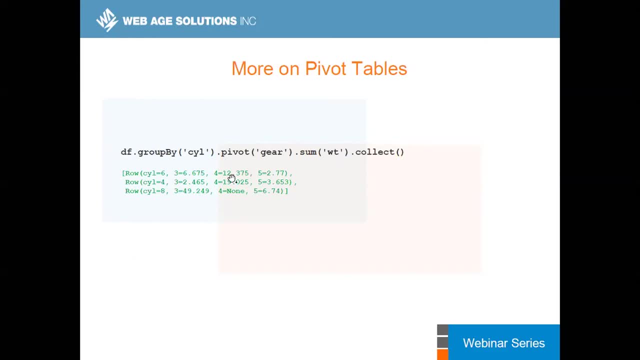 you to build a pivot table where, instead of the counts, every cell in that tab in the table- like virtual table which would be converted into a data frame- would collect the sum of weights of this car. and we see that by just looking at the data, we see that the cars which have three gears 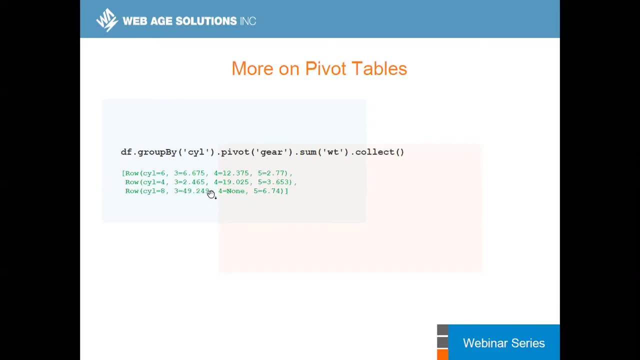 and eight cylinders are the most, the heaviest one, or maybe not the heaviest, but most of the cars are in this area. if we go to that table, yes, we've got 12 cars in this space. pretty much we kind of collaborate data. there is some. 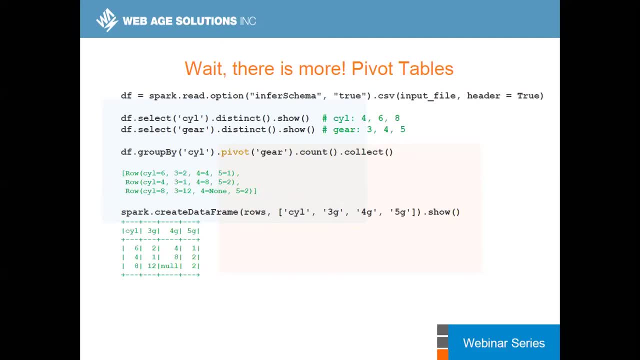 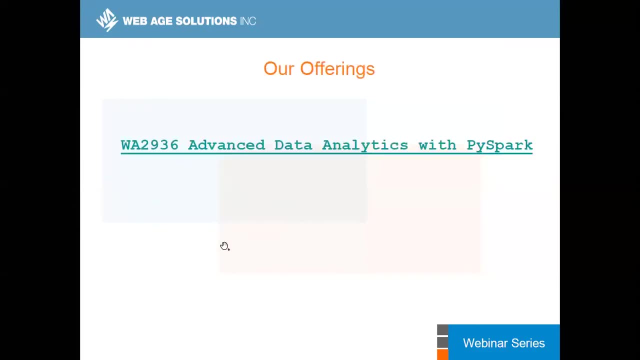 some sort of correlation between the count and the weight, right? so that's what I guess was the point. of course there is more, and definitely it wouldn't be possible to cover everything that we talked about here so far. usually there are more questions, right, and so that's the material that we offer. 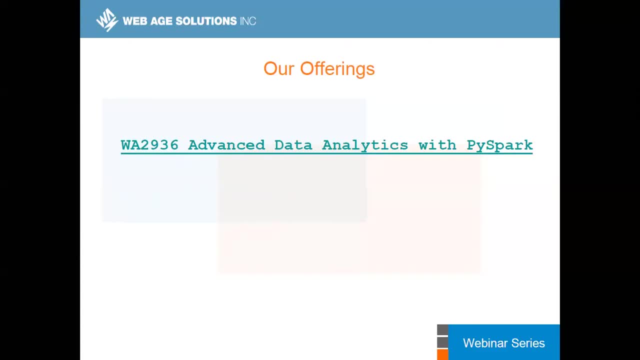 our clients. it's a two-day class which just has lots of hands-on. you just be touching on theory a little bit and then spending time and you will explore data frame api inside out. the lab environment is staged in beta bricks cloud. you will also have exposure to this environment so that 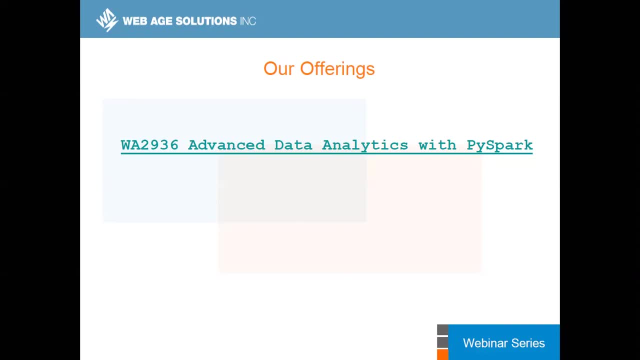 you can immediately. there's no delays, by the way, it's free access. you can start experimenting with your data so that you can get output. you will get instant return on your investment of your time. so after two days you will be able to start processing data, not using only sql, but also, more generically, the data frame api. so that's all for me. for 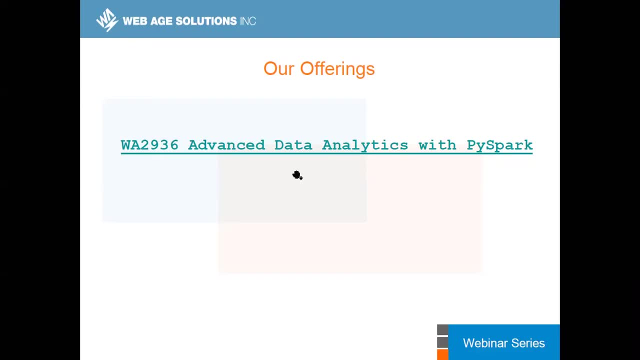 the day. I haven't heard from our people at the background office. maybe there are some. we kind of experienced some problems with some of the parts of organization being shut down due to that situation in the health department. so we still have a couple of minutes left before we. 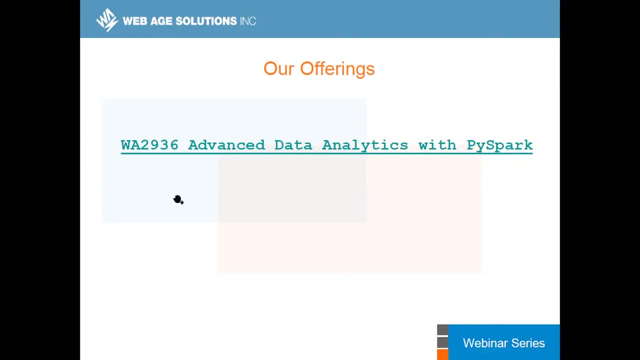 end this meeting. any questions? uh, so the question is: what is the best way to practice spy spark for free? as I said, uh, data bricks community cloud right away, instant. you just need to provide your working email and uh, they are very proud of what they're doing. they're not going to. 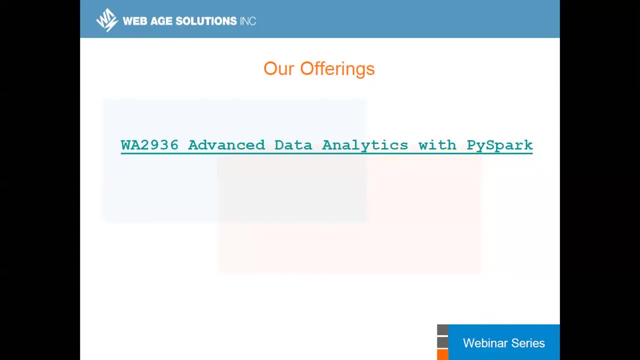 ask you for credit card number for your mother's maiden name, for for anything else, just provide email. you get the feedback. they pretty much are so confident that you will be, uh, continuing to work with them and eventually you will upgrade to a production production license so you can. 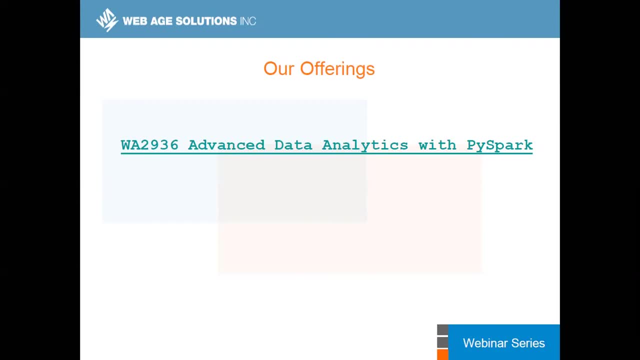 experiment it for free. that would be the best way I can suggest. if you kind of are more inclined to do things in a hard way, uh, download the spark standalone and start doing things there. it'll be a little bit more of a headache, really. other questions: uh, I mean to e-learn. 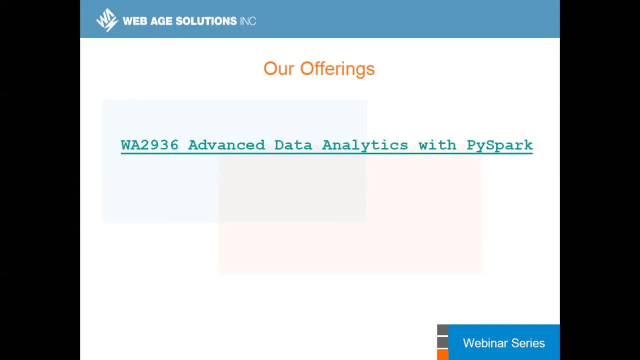 I'm not sure what the best way to practice spy spark is, but I think it's the best way to practice spy spark. um, this class is offered uh for um, as it it's not really coded right. um, I'm not sure what would be the best class. uh, it depends, um, on your background. uh, there is no answer that fits all. 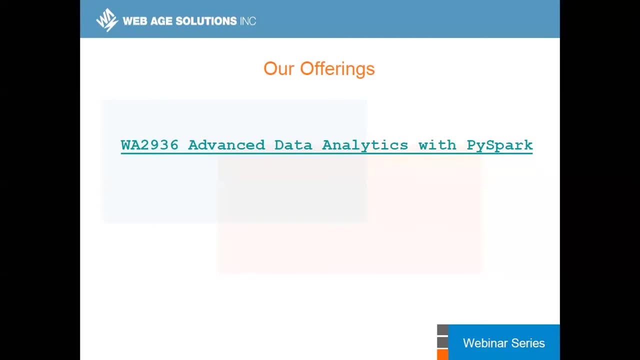 questions. no, I cannot answer, so, um, I guess try, I don't know. there's so many classes out there, um, plural side, I don't know, go there and whatever is currently, uh, it's always a place. but what I would like to tell you that all those classes, uh, they give you some sort of pre-recorded